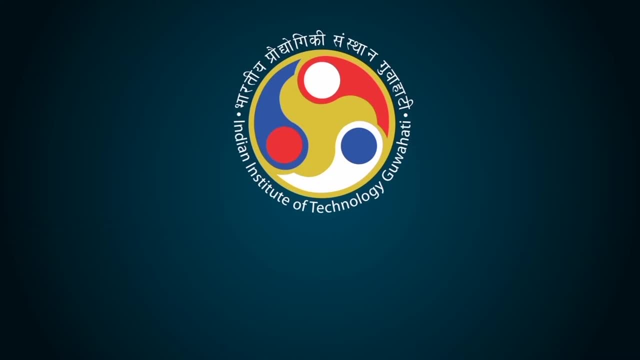 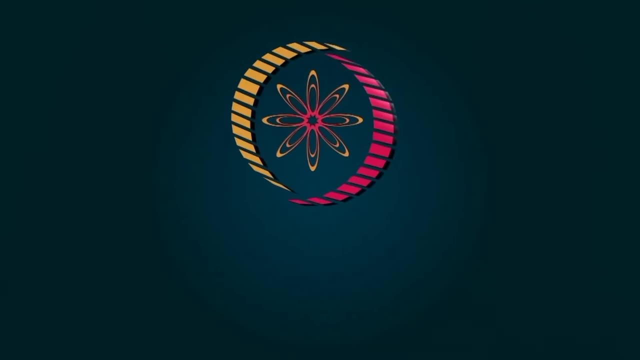 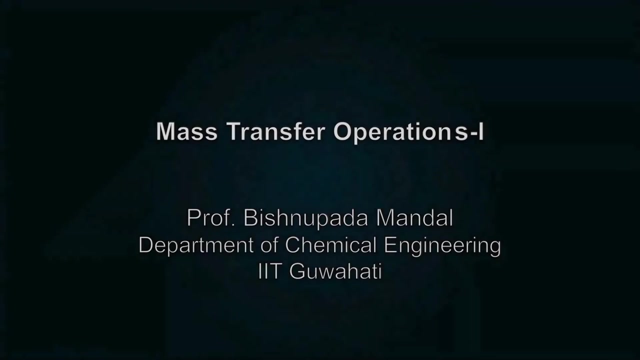 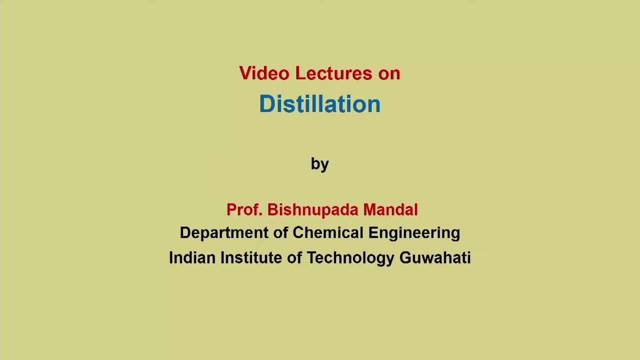 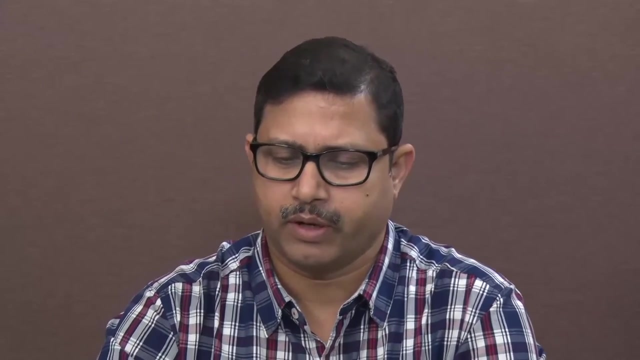 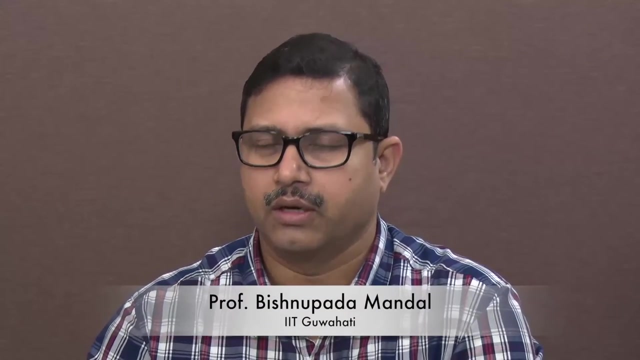 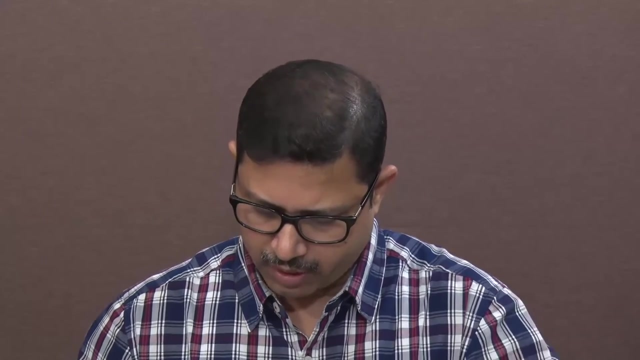 Thank you for watching. Welcome to 10th lecture of module 5 of mass transfer operation. In this module we are discussing distillation operation. So before going to this lecture, let us have a recap on our previous lecture. In our previous lecture we have discussed mainly two things. One is: 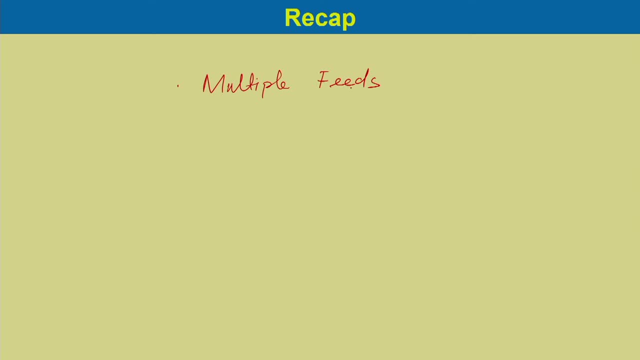 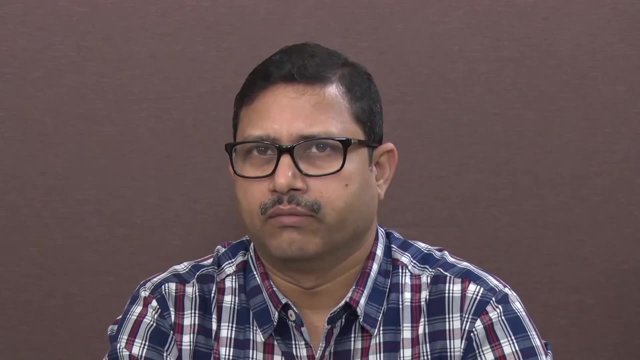 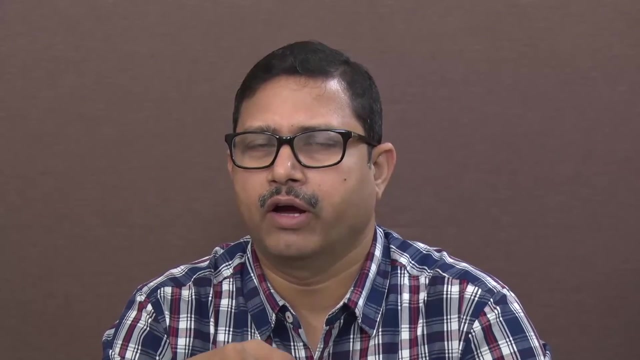 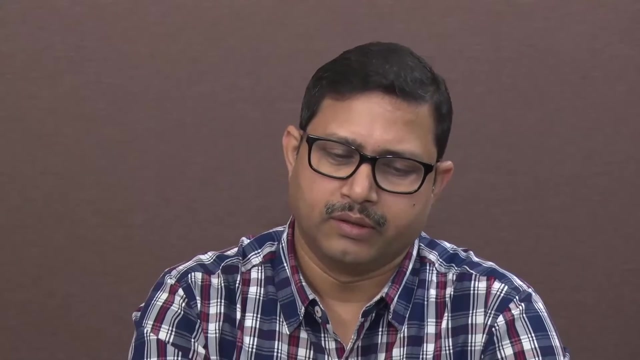 multiple feed. So for multiple feeds, we have seen how to obtain the different operating lines for different sections and how to calculate the number of ideal stages requires using the operating line and the equilibrium line. The second thing we have considered in this case is the multiple product withdrawal. 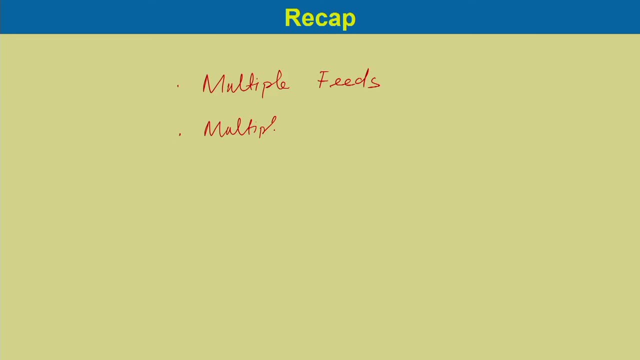 So this is also unlike in case of multiple feeds. we have the number of stages required and then feed plat locations we have determined. but in case of multiple product withdrawal, we have also seen how to calculate the number of igual accordingly. So, like in case of 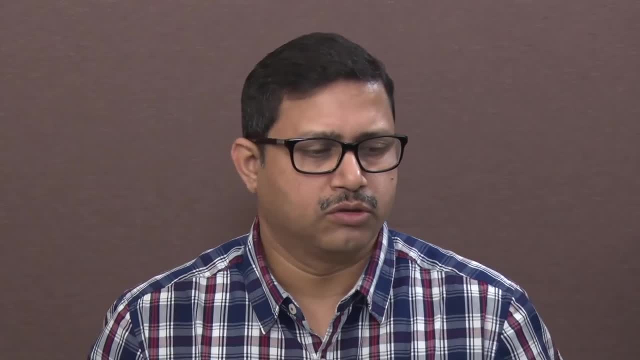 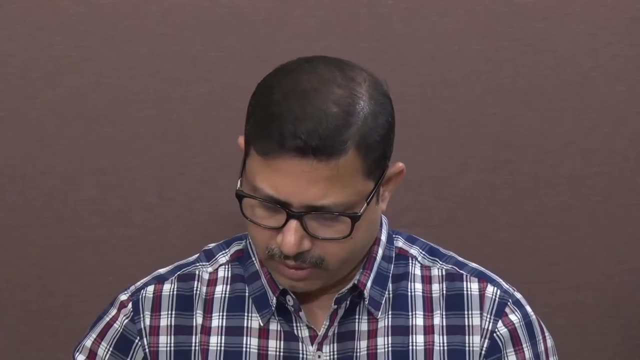 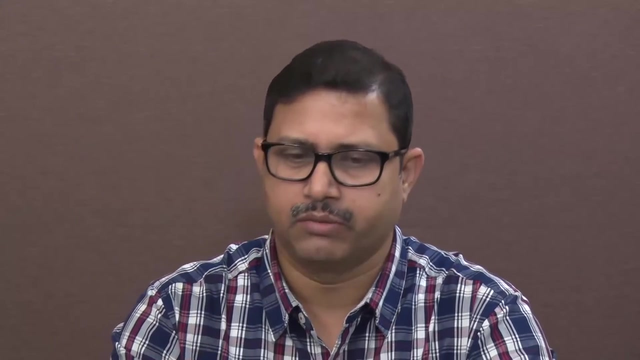 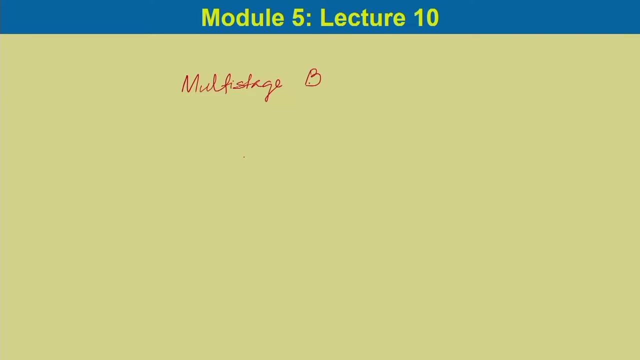 multiple feeds. we have the number of stages required and then feed plat locations. we have ideal trays from where the product is withdrawn. Now, in this lecture, we will know mainly discuss one important thing, which is, you know, multistage batch distillation with reflux, So earlier, 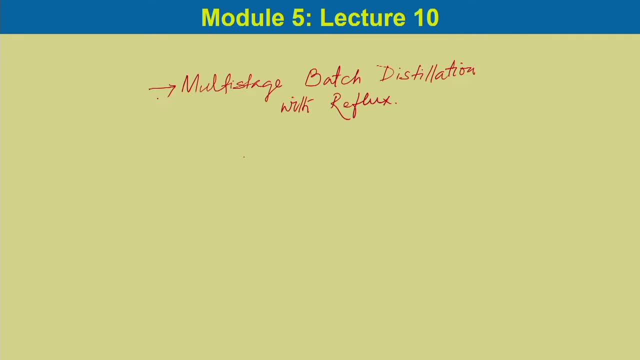 we have discussed, you know, multi, you know batch distillation with reflux, Now without reflux, in this case. now we will discuss batch distillation with reflux, under which we have two different condition: one is constant reflux and second thing we will considered variable reflux. 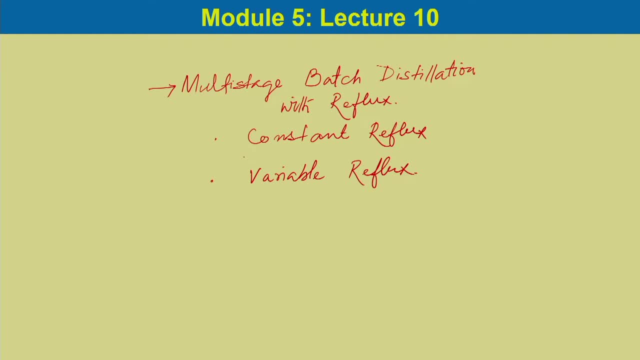 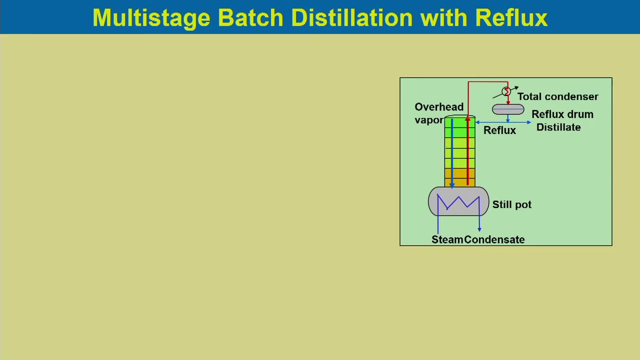 So multistage batch distillation with reflux. So you can see, in earlier case we did not had any reflux into the batch distillation column, So we had a steel pot and you have a different stages in the column and then there is a condenser. 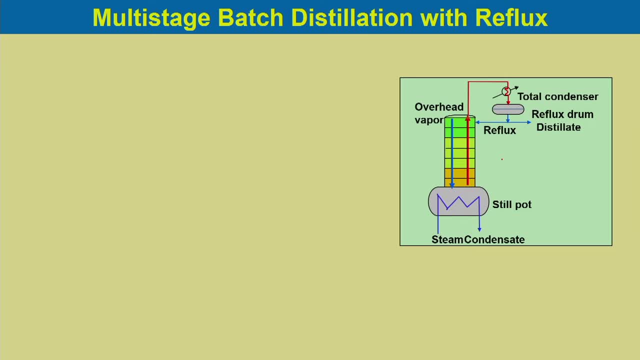 and then reflux drum and you have a reflux ratio you can control and you can get the product outlet at the top You just tell as a distillate. So in single stage, batch distillation, that is Rallye distillation, which we have discussed before, the purity of the product is practically governed by 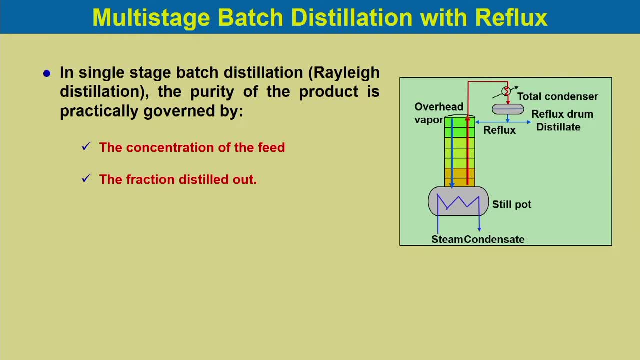 the concentration of the feed and second thing is the fractions distilled out. So these two parameters, the concentration of the feed and the fraction distilled out, this will determine the purity of the batch distillate. So it is seen that we had less. 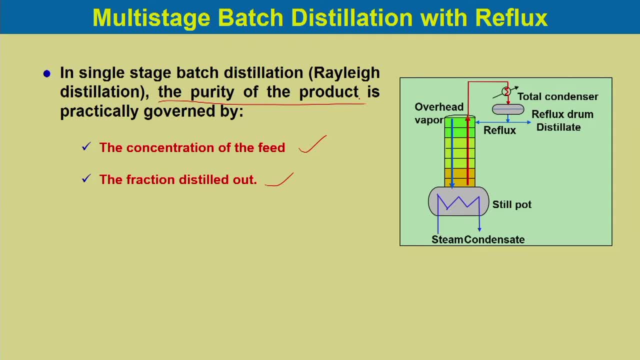 filtering Rabshainite in this distance. So you have seen that this crossing is Purity of the product you are getting in a single stage distillation unit. we call it no Rayleigh distillation. However, if a batch liquid is distilled in a multistage column, 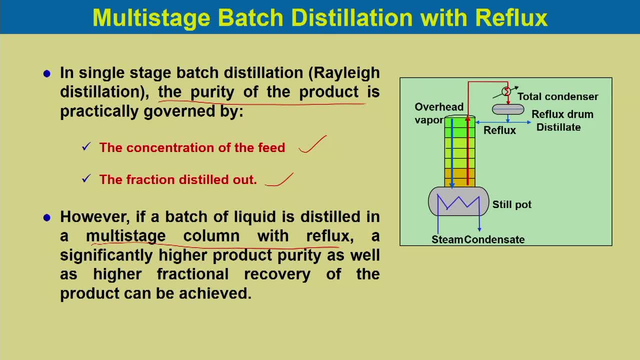 with reflux. a significantly higher product purity as well as higher fractional recovery of the product can be achieved. If we use the multistage instead of single stage, and if we also control the reflux or if we give the reflux back to the batch distillation column, we could achieve higher purity of the product and also the fractional recovery of. 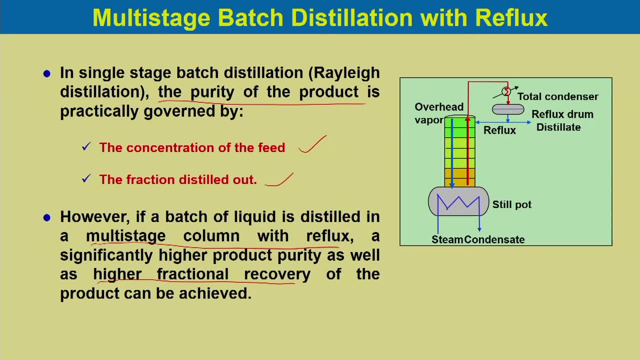 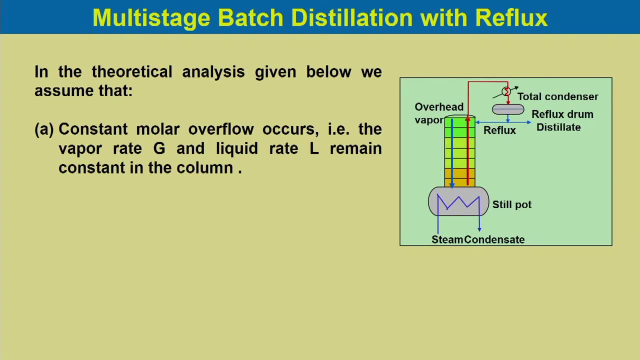 the product of the solute will be increased. In the theoretical analysis given below, we assume certain things. one is constant: molar overflow occurs. that is the vapour rate G and the liquid rate G. The vapour rate L remains constant in the column. So that is the first assumptions. 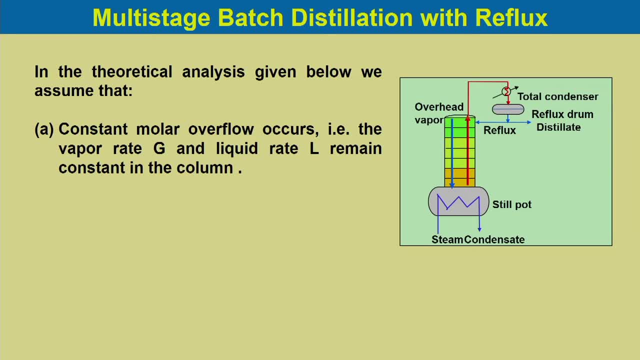 we will do for the theoretical analysis of multistage batch distillation. with reflux Liquid holdup on the plates is very negligible. and third thing, we will assume batch distillation is an unsteady state process. but in this case we assume that the pseudo steady state 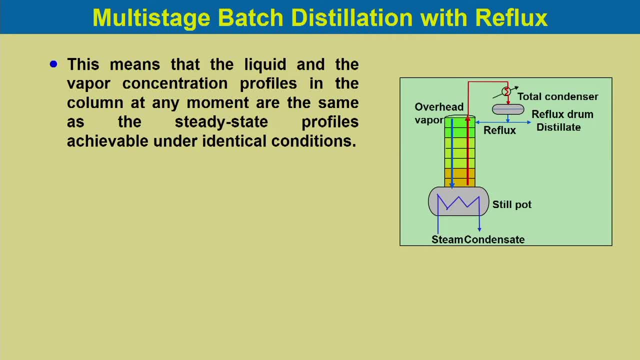 condition prevails, That means the liquid. The liquid and the vapour concentration profile in the column at any moment are the same as that the steady state profiles achievable under identical conditions. So we call it pseudo steady state condition, which prevails in case of batch distillation with reflux. 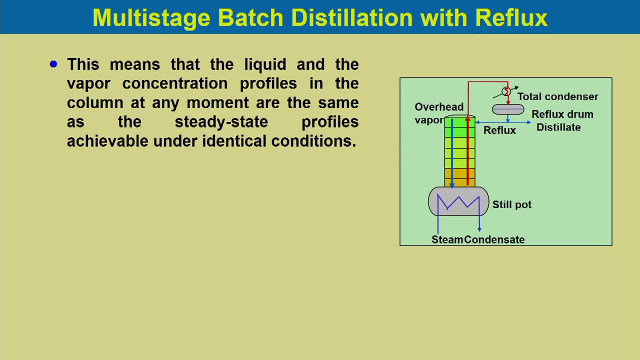 for a multistage batch distillation column. It is easy to understand that if the reflux ratio is held constant then the Jason boundaries will be not stable. So for a batch distillate held constant, the distillate concentration will decrease as the distillation proceeds. 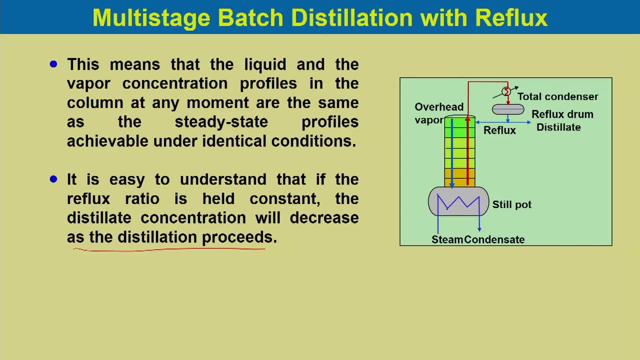 Because, as you know, initially in a batch distillation column, when the, you know, still the still pot is heated, of the solution or the mixture, the more volatile component will be rich, much richer in the distillate. So the initially the product concentration will be much higher. 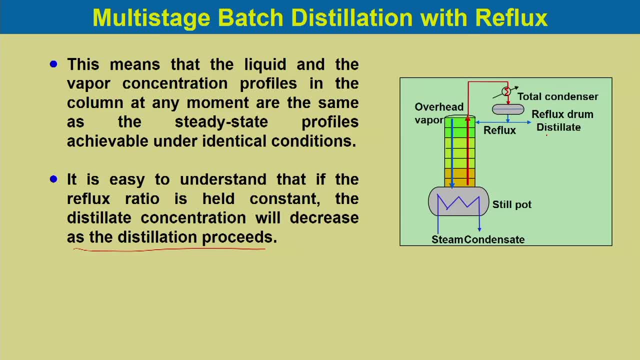 of the more volatile component at the top. As long as the distillation will proceeds, the composition will gradually change and more of the less volatile components will also mix, because the still pot contains less quantities of the more volatile components. So as long as the distillate is rich, the distillate concentration will be higher and 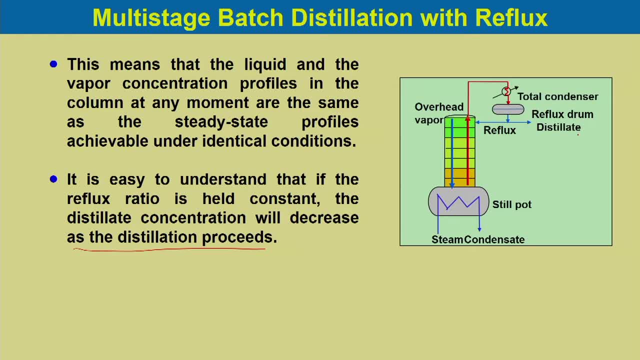 the of the solution will decrease. So this is the composition of the distillate, and the distillation will proceed. the composition of the solute concentration will decrease, So the column may be operated till the distillate quality remains within the acceptable limits. 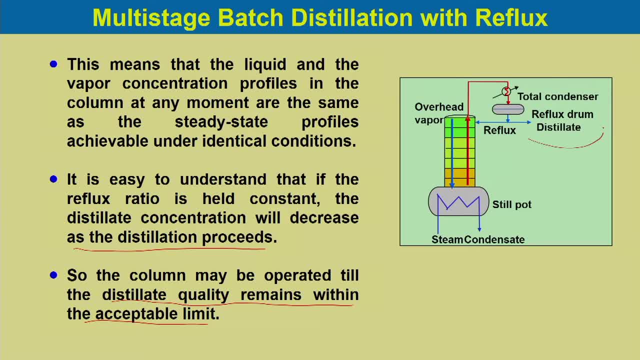 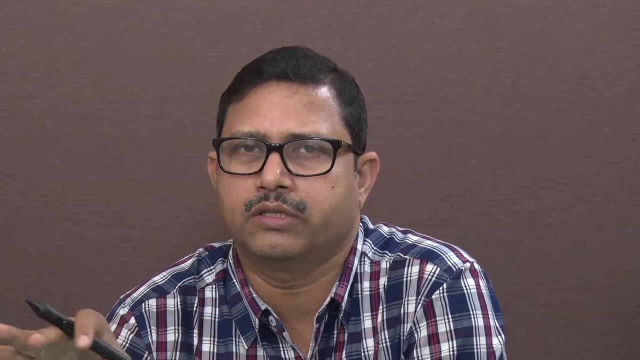 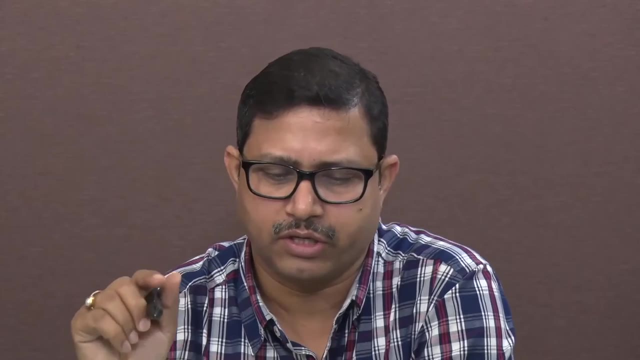 Depending on our requirements of the average composition of the distillate, the product composition we need for the solute or more volatile components. until, unless it is within the acceptable limit, we can continue our distillation and we stop where the quality desired quality is required. So until that period, we can operate the distillation for a fixed reflux. 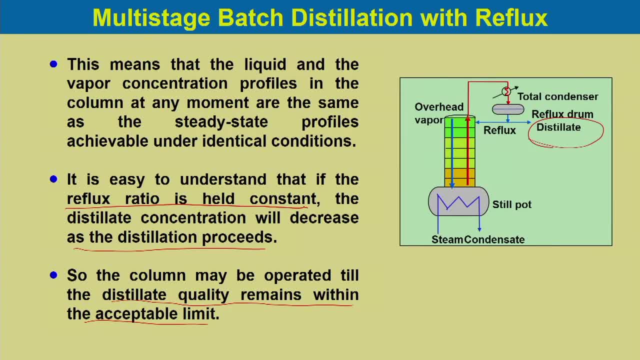 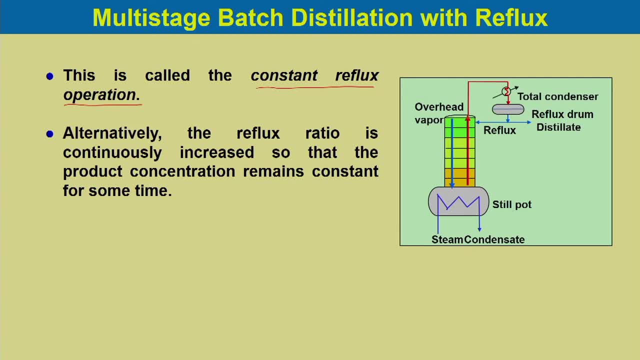 ratio or constant reflux ratio. this is called the constant reflux operation. Alternatively, what we can do: the reflux ratio is continuously increased so that the product concentration will decrease, So this is called the constant reflux operation. So this is called the constant reflux operation. So what we can do if we want to have a high purity. 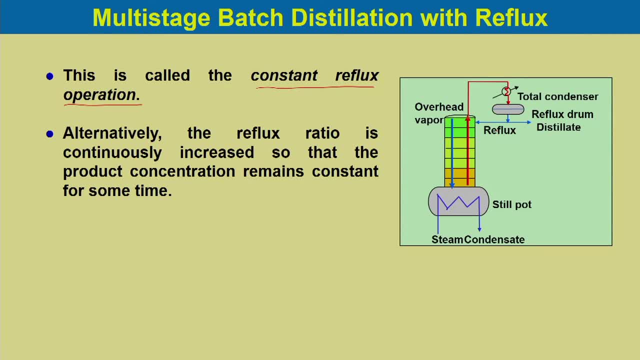 product at the distillate we can change the reflux ratio from very low to very high. So reflux ratio will be changed in such a way that the product concentration does not change for a certain period of time. this is called variable reflux operation. 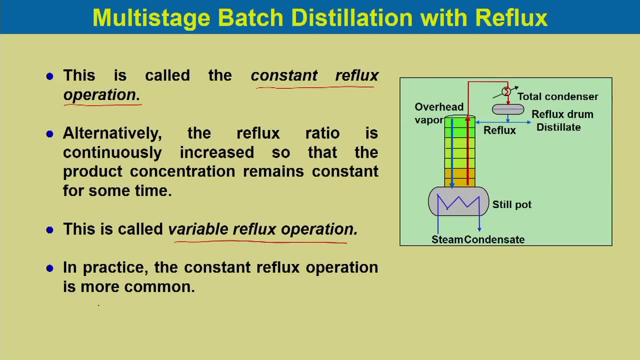 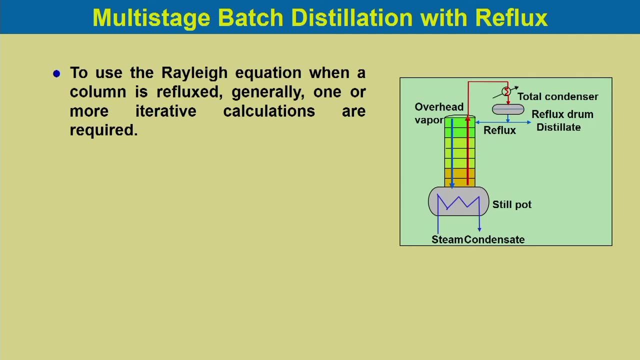 In practice constant reflux operation is the more common. So constant reflux ratio operation is very easier to you know operate and that is most common in case of multistage batch distillation with reflux. To use the Rayleigh equation, when a column is refluxed, 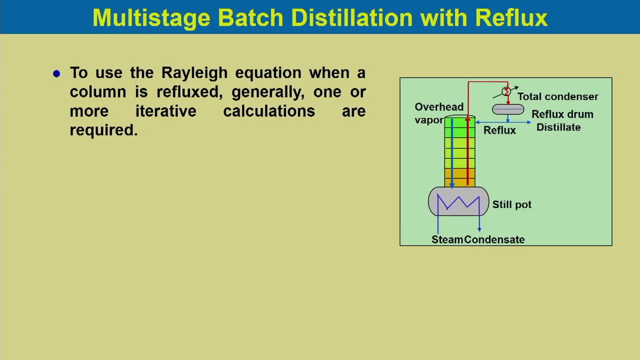 generally 1 or more iterative calculations are required. So to calculate the- you know- minimum number of trays that are required, then we have to do an iterative calculation of trays required for a no particular separation. if we want to use the Rayleigh equation, then 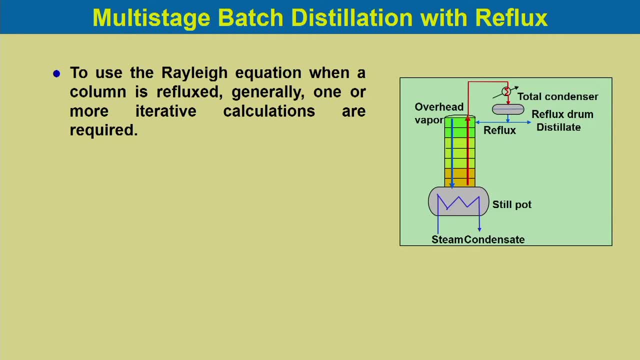 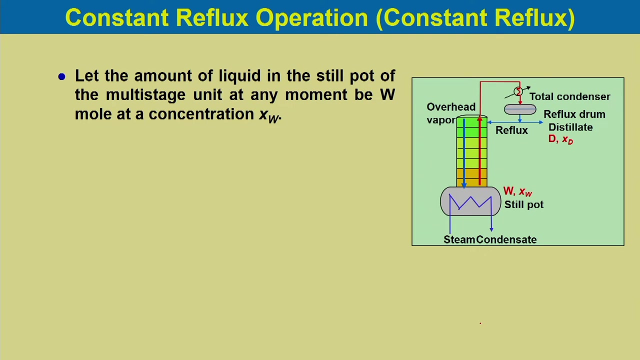 we have few iterations, which would be required for the multistage batch distillation with reflux. Typically, a McCabe-Thiele diagram is used to obtain some of the information needed in the calculation. Now let us consider the first case: constant reflux operation. that is constant reflux. So reflux ratio remains constant. So the 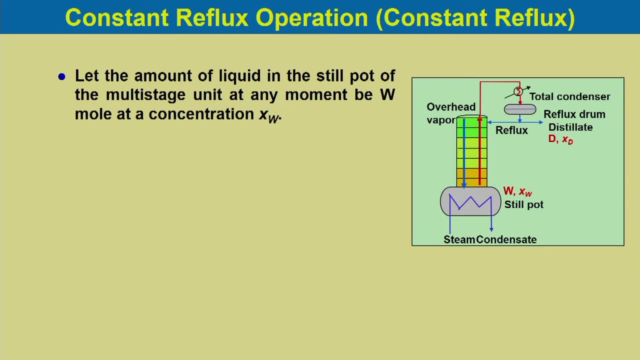 product concentration will gradually change and let the amount of the liquid in the steel pot of the multistage unit at any moment be W mole and at concentration, x W. So this is the concentration, So this is the concentration. So this is the concentration, So this is. 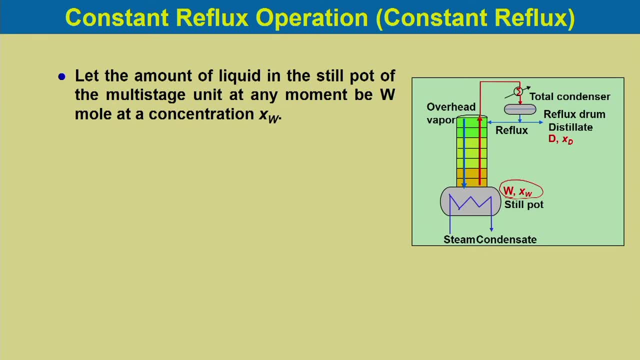 the total number of mole at any time. t W is the mole in the steel pot and you know x W is its mole fraction, the more volatile component, x W. Over a small time, d d mole of distillate is withdrawn and the amount of the liquid in the steel pot decreases by. 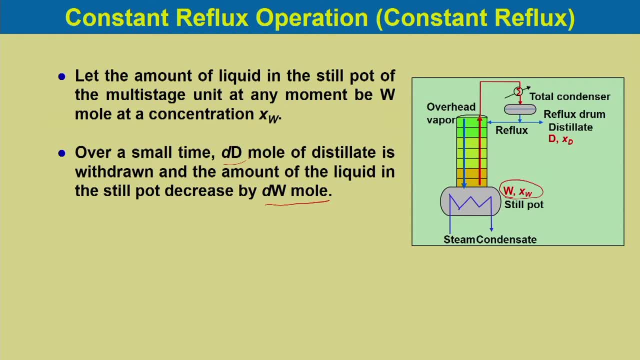 d, W mole. So the amount of distillate we withdraw at this location, same amount of liquid which will decrease in the steel pot in a very small time, d t. So we can write from here: minus d, W, x, W would be equal to x, d, d d, which would be equal to. 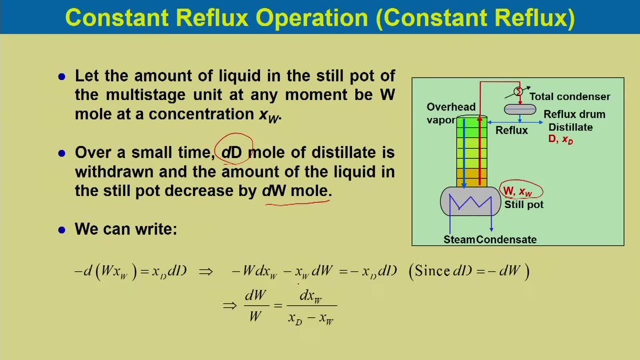 minus W d x W. So this is the concentration. So this is the concentration. So this is d x W minus x W d W would be equal to x d d d, which is equal to no minus x d d W, because 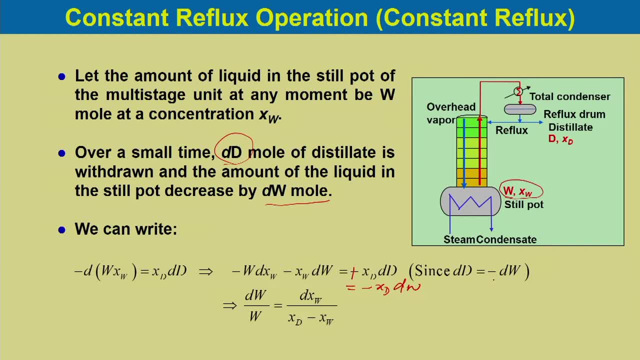 d d is equal to minus d W. So if we simplify this, from here we can write x W into d W minus x d d w would be equal to minus w d x w. So from here we can write x w minus x d into. 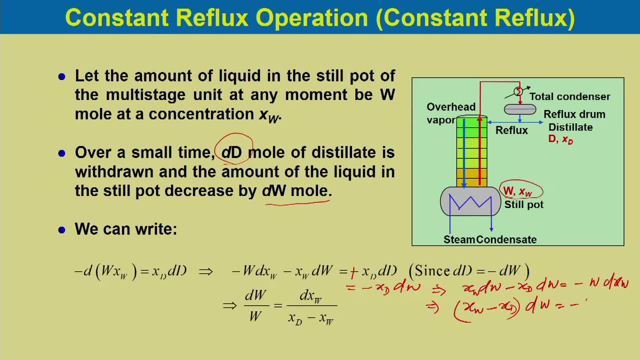 d w would be equal to minus w d x w and we can write x d minus x w d w would be equal to w d x w And from here we can just rearrange. we can get d w by: w would be equal to d x. 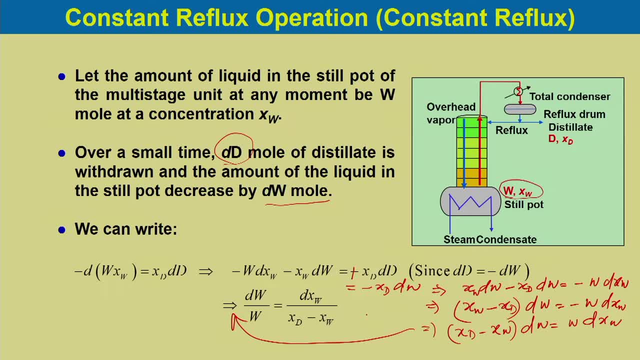 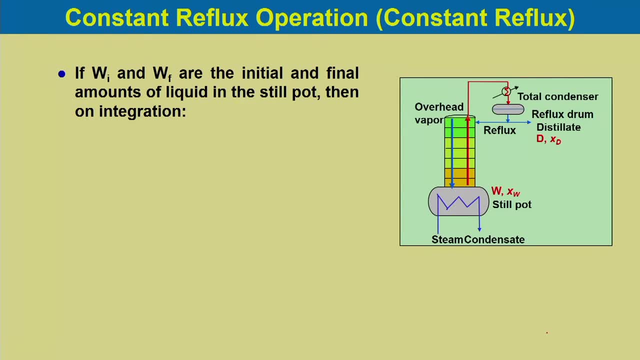 w by x w. So now, if w i and w f are the initial and final amounts of the liquid in the steel pot, then on integration we can get ln. w i by w f would be equal to integral x w, f, x w i to. 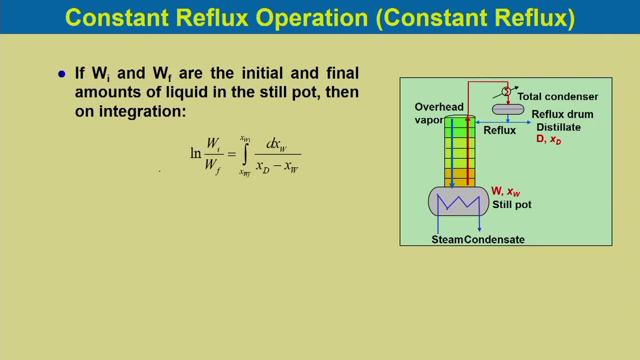 d x w by x d minus x w. So this is the integral form of the equation, where the composition changes from x w i to x w f As the distillation proceeds. x d and x w both keep on changing, So both on the 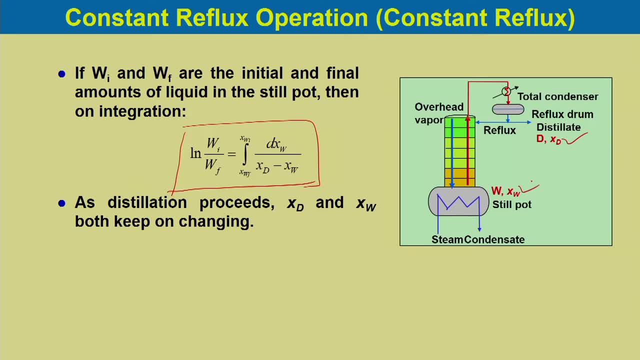 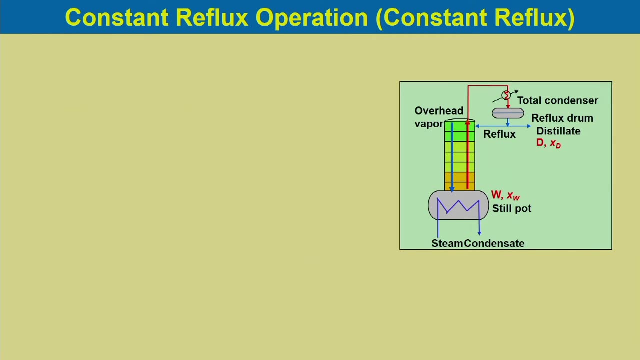 distillate, x d and at the steel pot, x w. both are keep changing in the batch distillation as the distillation proceeds. So the integral in the above equation, in this equation can be, you know, evaluated graphically. So of the four quantities, that is, w i, w f, x w i and x w f, any one can be calculated. 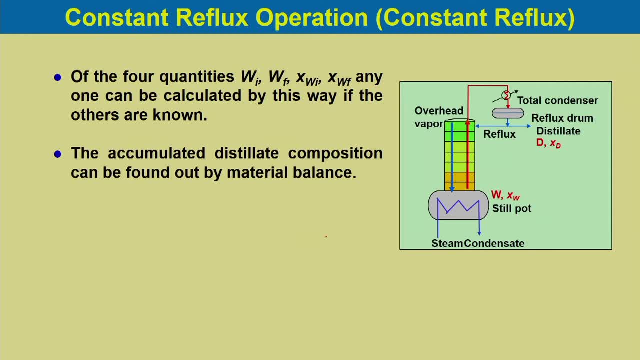 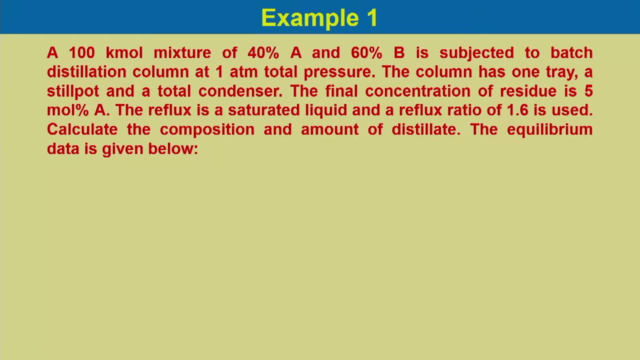 by this way if the others are known. So the accumulated distillate composition can be found out by the material balance. This is the column at one atmosphere pressure. The column has one tray, a steel pot and a total condenser. The final concentration of the residue is 5 mole percent A the reflux. 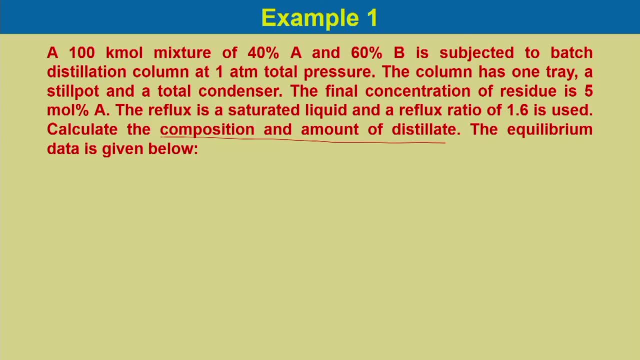 is a saturated liquid and the reflux ratio of 1.6 is used in this case. Calculate the composition and amount of distillate. The equalband of постоянно inflow, say cetera Ş, is equal to the distance difference island or a أ of the flow between arc and beam. 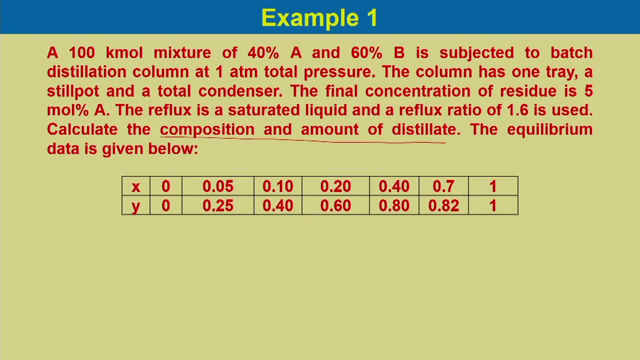 if itOOO exists, it is equal to this ratio. So it is8 by 0.7. and if it os 1 is less than 0,0, ήταν equilibrium data is given, So x and y data are given, So we can plot the equilibrium. 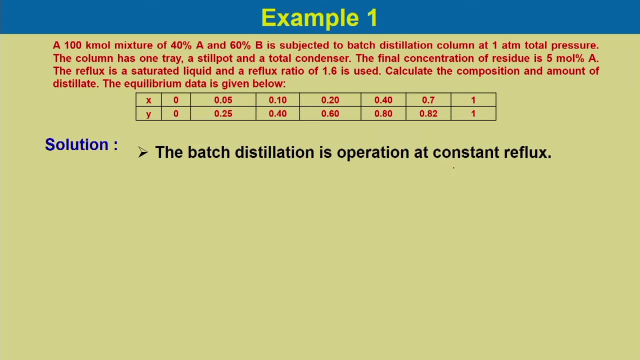 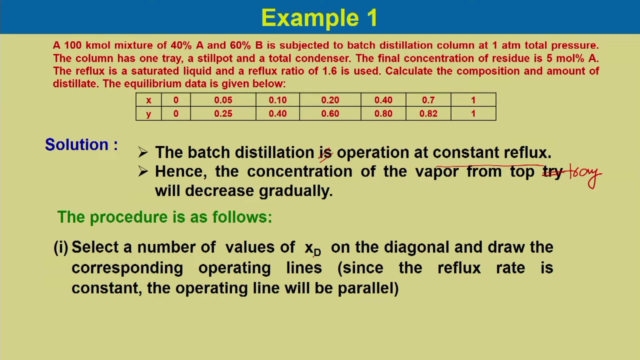 curve, So the batch distillation with constant reflux, hence the concentration of the vapour from top tray, will decrease gradually. and the procedure to be followed: select a number of values of x, d, that is, the no distillate product on the diagonal, and draw the corresponding 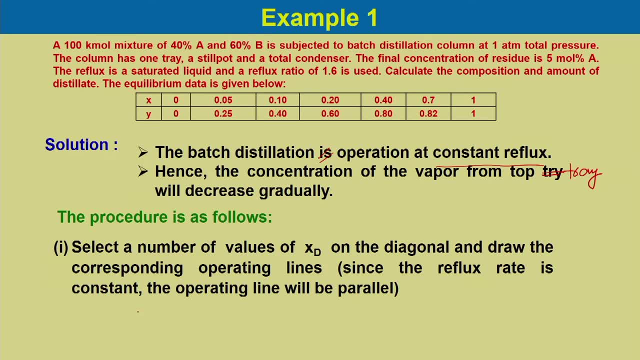 operating lines. Since the reflux rate is constant, the operating line will be parallel because R is constant. So the slope of the operating line R by R plus 1, this slope remains constant. Since the reflux ratio is given 1.6, we can: 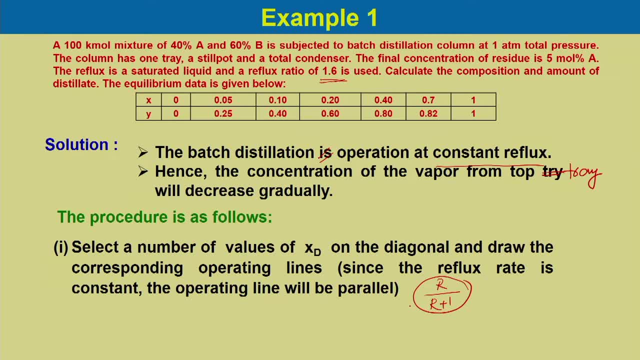 plot it. So the procedure is to select any point on the 45 degree diagonal and draw at different points on the 45 degree diagonal, that is, x, d, and then we can plot the parallel operating line, because the slope are same For each values of x, d. determine the value. 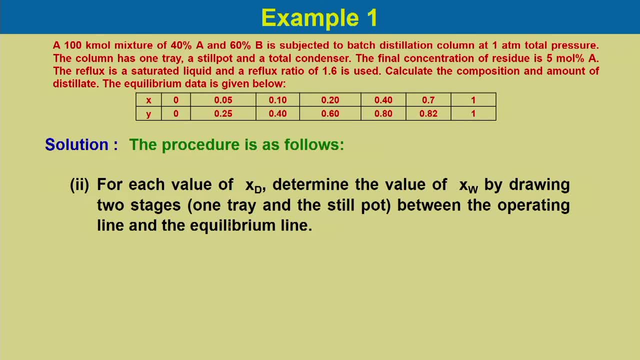 of x- w by drawing two stages, one tray and the steel pot between the operating line and the equilibrium curve. So we have one tray and one steel pot. If, from the operating line to the equilibrium curve, if we plot two stages, then we can get the values in the steel pot. 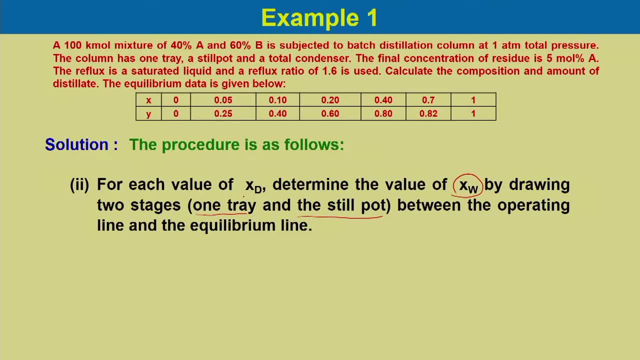 which is x w. So for a particular values of x d, we can calculate x w. Thus we shall have a set of values of x d and x w with the concentration range of x wi, that is 0.4. initial concentration, which is 40 mole percent A, and the final concentration. 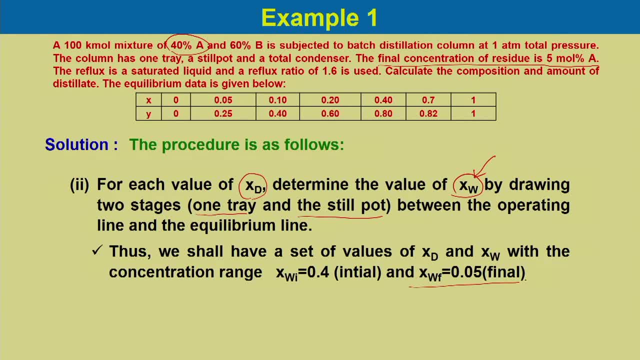 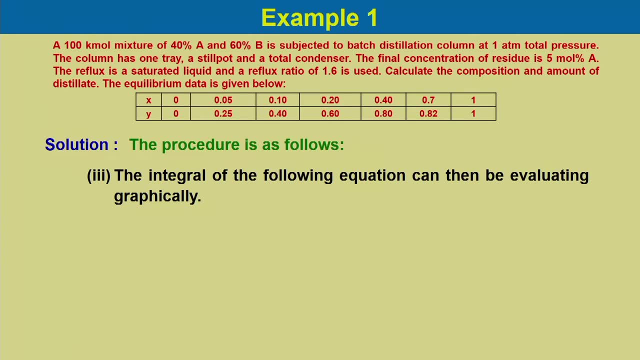 of the residue is 5, mole percent, it is 0.05.. So this is the final x, f, x, w, f. So the integral of the following equation can be evaluated graphically. So this is the equation. So we have set of values of x, d, x, w. 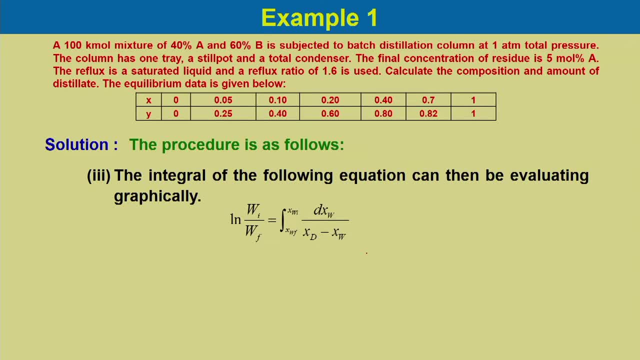 And from there we can calculate 1 by x d minus x w and we can calculate the area under the curve graphically to get the integral values of this. So the reflux ratio R is 1.6, which is given. So slope of the operating line R by R plus 1 would be 1.6 divided by 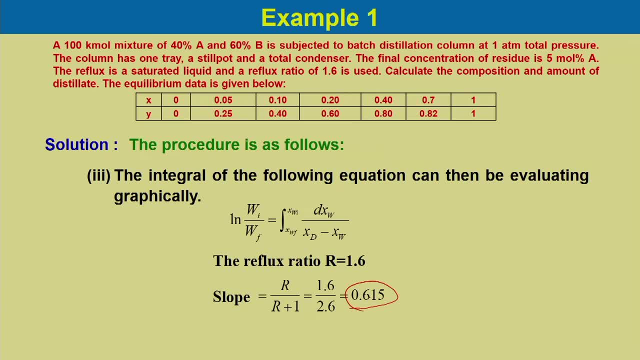 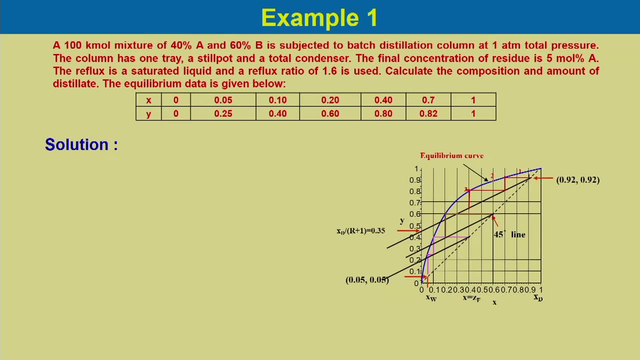 2.6.. So 0.615 is the slope of the operating line. You can see over here. So this is the equilibrium curve which is given over here and you select any point. it is taken from 0.9292,. but actually if you just plot the equilibrium line and 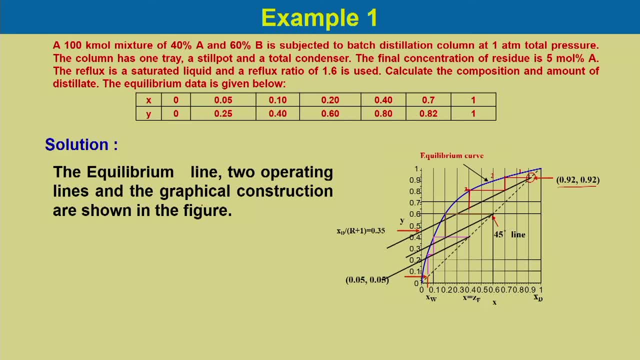 then two operating lines, both the stripping section and rectifying section. you need not to draw the operating line for both the sections. So from here with the slope you plot operating lines. So once one operating line is known, so other operating line you can draw from the 45 degree diagonal by drawing the parallel. 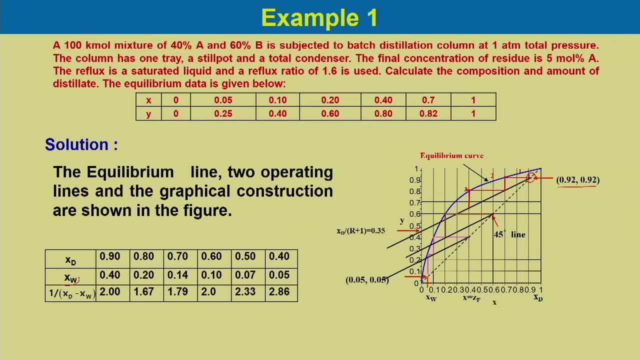 lines We have to come to the initial concentration, that is, x w. So we will choose the x d in such a way that we can obtain x w, which is 0.4, at the initial concentration in the steel pot. So when x d is 0.9, if you plot two trays you will get the concentration of x. 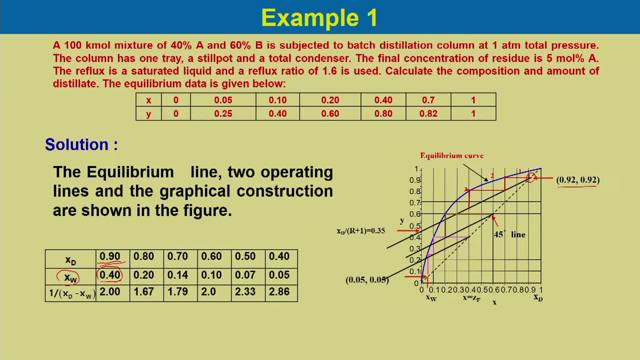 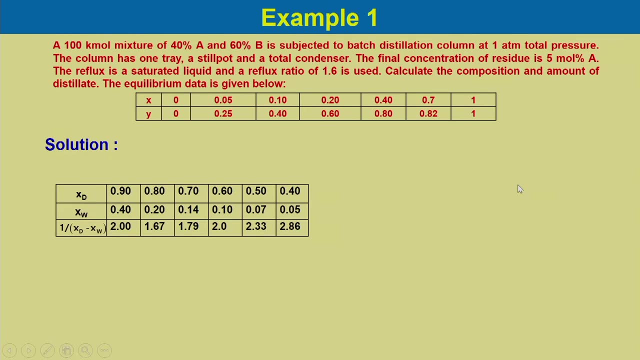 w as 0.4.. So basically, you start from a point here and then go to the equilibrium line and then from here you go to the operating line, go vertically to the operating line and then go horizontally to the equilibrium curve and corresponding to that. So this is the equilibrium curve and corresponding to that you can draw: 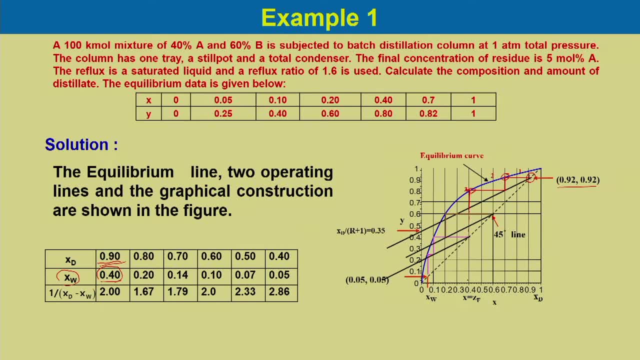 you will get the values of know. go to the x axis, which is know around 0.35 with respect to 0.92, if you take a know point at 0.92 and with the slope of the operating line 0.615.. 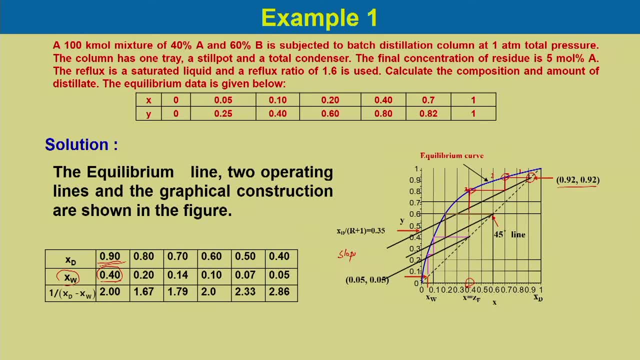 So slope is equal to R by R plus 1, which is 0.615.. Right Right, Right, Right, Right, 615, because R is equal to 1.6, and if it is 0.92 it intercept at 0.35 X D by R plus 1.. 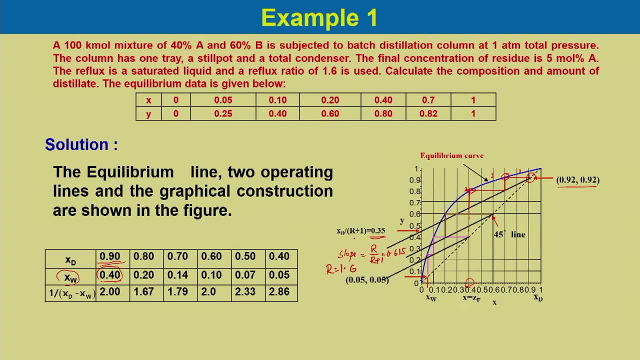 When the X, D is changes and reflux ratio is constant. so you will have a different cut and you will obtain the values of know. for two columns you will obtain the values. So the similar procedure which is shown over here for know 0.9292 and for other know X. 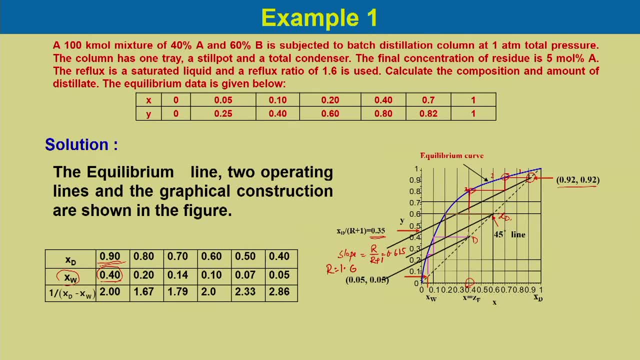 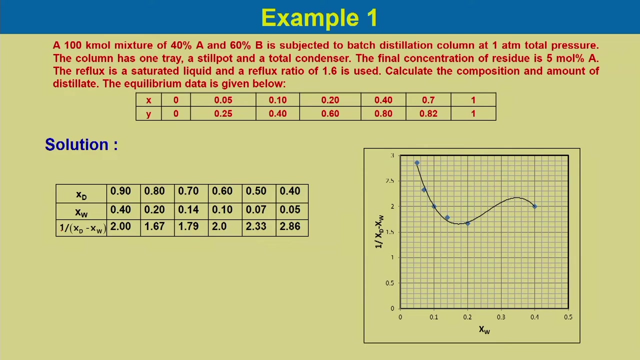 D values, different X D values. So X W obtained X W from 0.4 to 0.05.. So this is the X W F and this is X W I and corresponding X D. you can know you have corresponding x d is 0.9 and 0.4, x d and x w known to us. So we can calculate 1 by x d minus x w from. 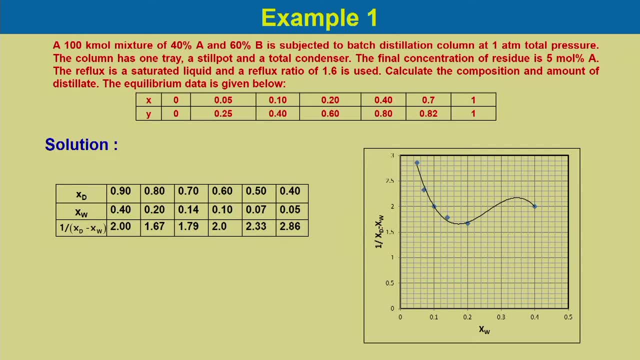 this data and we can plot 1 by x d minus x w versus x w, as shown over here. this is starting from 0.4, that is, x w up to 0.05.. So which is over here, so middle of this? So x w is. 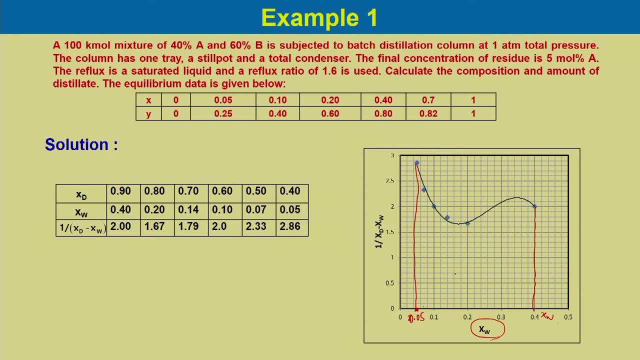 it is 0.05.. So the area under the curve you can calculate. use different methods to calculate the area under the curve, either trapezoidal method or trapezoidal method, Or Simpson one third rule or some other method to calculate the area under the curve. So 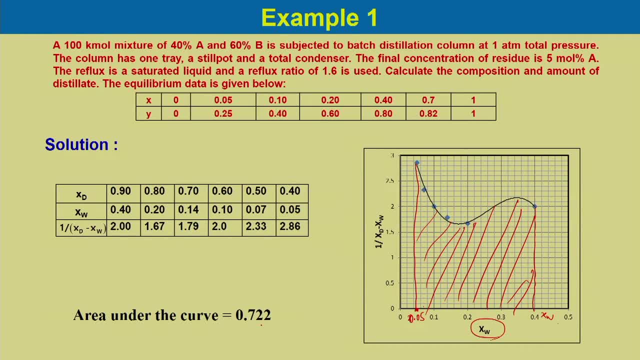 the area under the curve would be around 0.722 if you calculate. So it is close to that and this is the equation: ln w i by w f is equal to this. So this is we have calculated which is area under the curve. 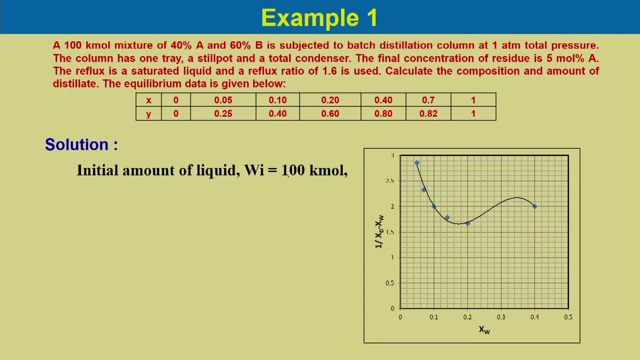 Now the initial amount of the liquid. The initial amount of the liquid. The initial amount of the liquid which is know W i, is 100 kilo mole. So if we use in this, in this equation, so L n 100. 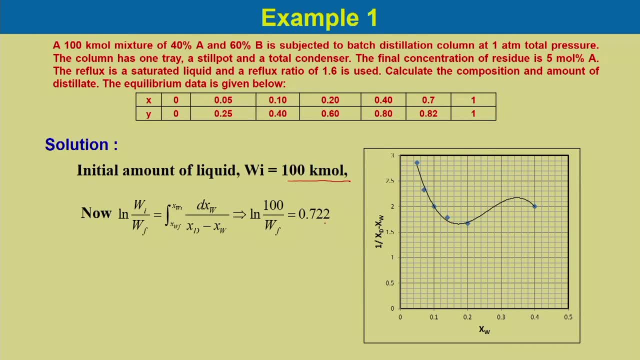 by W f would be equal to 0.722.. So from here we can calculate: W f would be equal to 48.59.. So final moles, which is on the steel pot, we can obtain this. So the distillate which 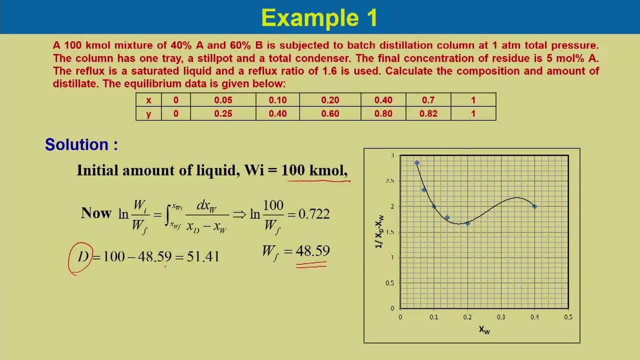 we got can be obtained from the total material balance equation, which is 100 minus W f, which is 48.59.. So it is 51.41.. And then the average composition we can calculate. the X D average would be equal to 100 into 0.4, 40 percent at the feet initially, minus 48.59. the final. 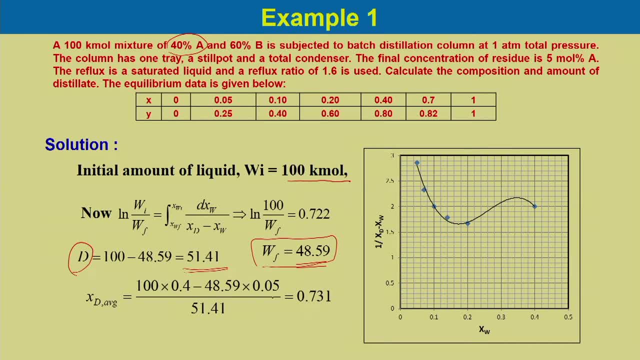 residue, which is 48.59 mole into W f. So W f into 0.05 mole fractions. divided by distillate, that is 51.41.. So it is 0.731.. So X D average is 0.731.. So this is how we can calculate the composition and the amount. 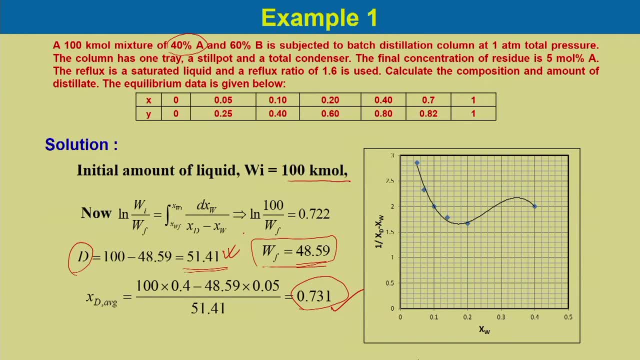 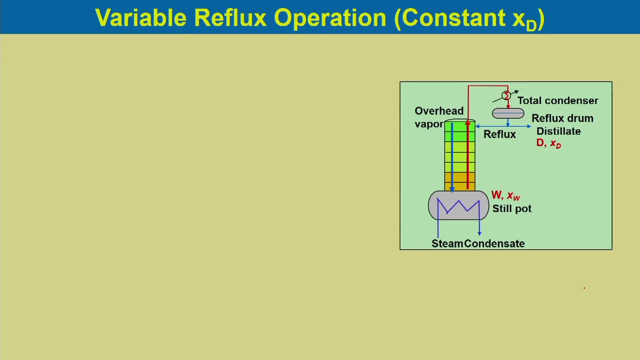 of distillate. So this is the composition and this is the amount of distillate. Now let us consider the another case, the variable reflux operation. So in the variable reflux operation we keep the distillate composition constant, that is, X, D is constant. So in a 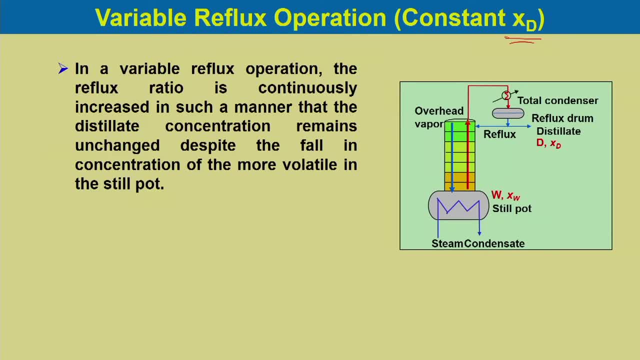 variable reflux operation. the reflux ratio is continuously increased in such a manner that the distillate concentration remains unchanged despite the fall in the concentration of the more volatile in the steel pot. So if the reflux ratio is varied, although the concentration on the steel pot over here, 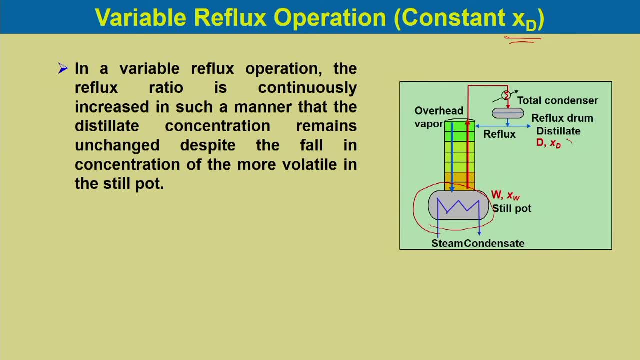 is changing continuously, but the distillate composition X D remains constant. Now if D G, D L and D D are the changes in the rates of the vapour flow, liquid flow and distillate withdrawal, So in that case we can write: D G would be equal to D L plus D D. So this is equation. 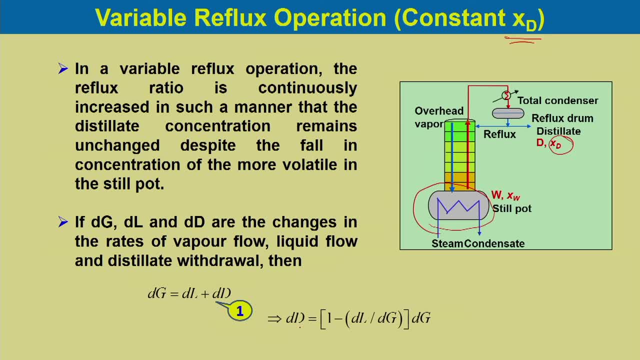 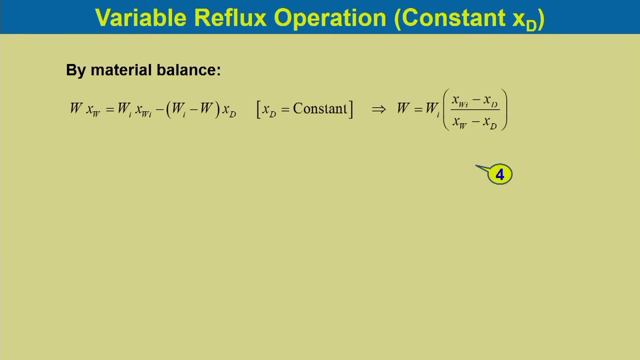 1 and from here, if we rearrange, it would be D D would be equal to 1 minus D L, by D G into D G. So this is equation 2.. So now if we do the material balance, So in this case Wx W would be equal to Wi, X Wi minus Wi minus W into X D, So Wi is the. 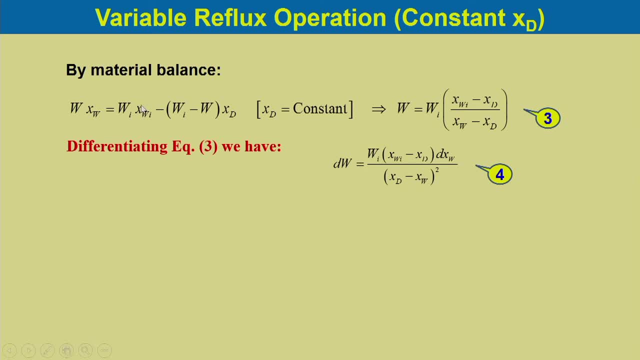 initial moles in the steel pot and its composition is X, Wi. W is mols in the steel pot and its composition is X, W and X. D is the distillate composition which is constant in case of the variable reflux. So by material balance we can obtain this relation. from here we can write: W would be. 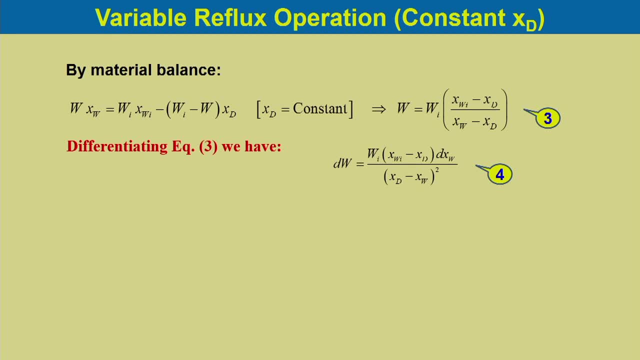 equal to W i X W i minus X d by X w minus X d. Now, if we differentiate this equation 3, we would obtain: d? W would be equal to W i X W i minus X d, divided by X d minus X w. 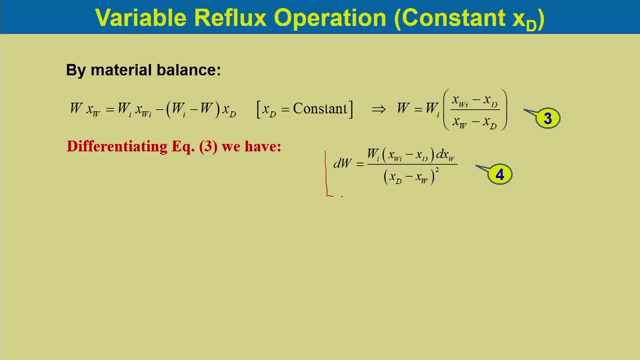 square into d X w. So this is the differential equation of the equation 3.. So this is equation 4, and if we substitute equation 4 in equation 2, equation 2 is this: one d d would be equal to 1 minus d L by d G into d G. d d would be equal to minus d W. 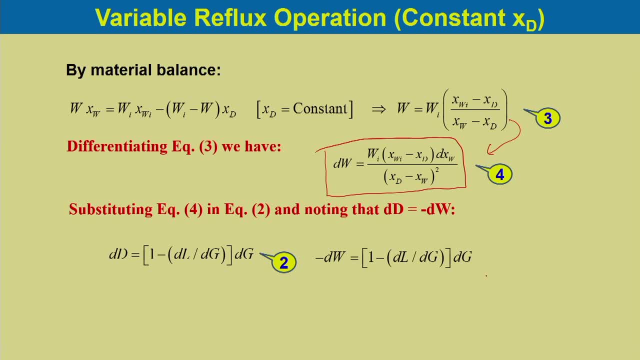 So if we substitute over here, in this case equation should be: minus d L by d G into d W would be equal to 1. minus d L by d G into d G. This is equation 5, and if we just substitute this one, d G would be equal to W i into X w i minus X d into d X w divided by X d minus. 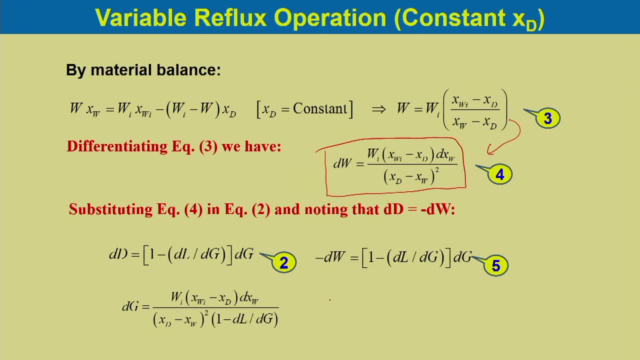 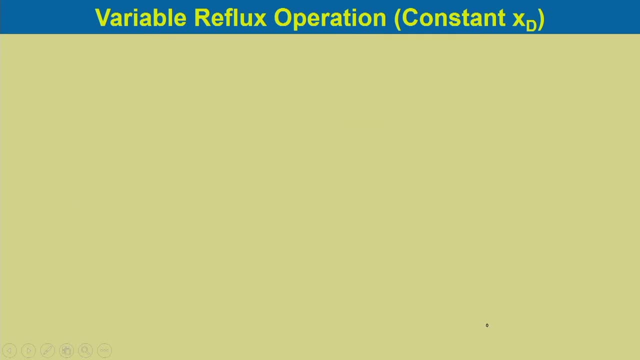 X w square into 1 minus d L by d G, So this is equation 6.. Now, if we integrate this equation right, So we can obtain the total amount of vapour generated from the steel pot. So during the 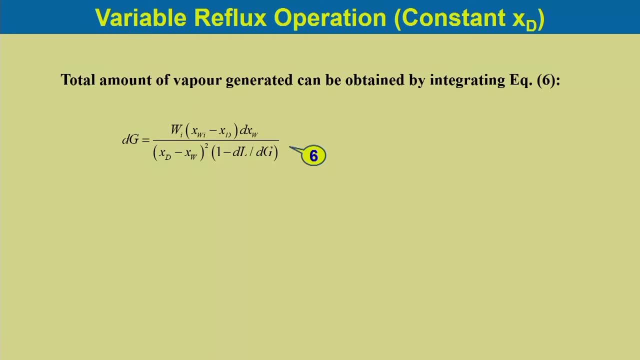 distillation, the amount of vapour which would be generated can be obtained by integration of equation 6.. So if we integrate, G would be equal to integral X w i to X w, f W i into X w, i minus X d, divided by X d minus X w square into d, X w square into d, X w square into d. 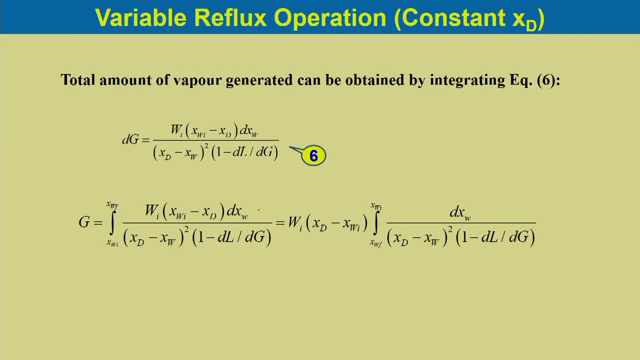 w square into 1 minus d L, by d G into d w, d x w, which would be equal to w i x d minus x w i, because these are the constant values initial and the distillate composition does not changes. this is the initial mould, So these are constant quantities we have taken. 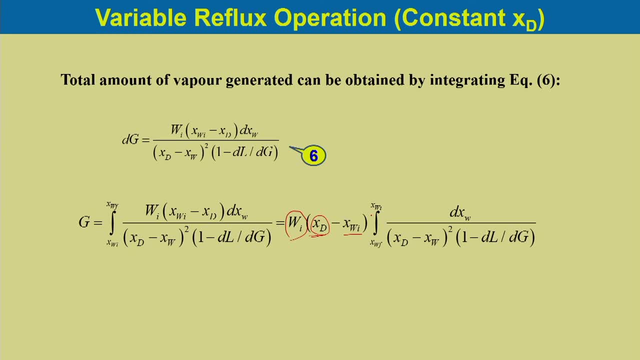 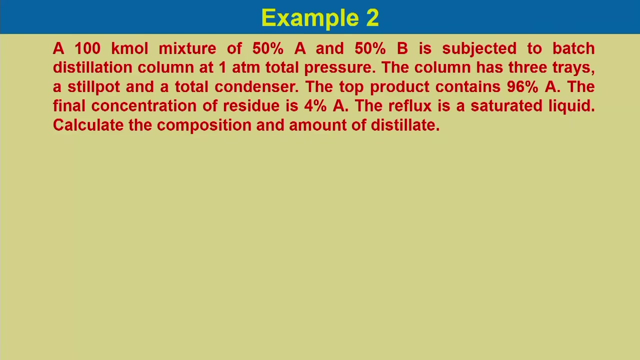 out from the integral and now this: we have to find out this integral. So this is equation 7 to calculate know the vapour generated in the know distillation process for variable reflux with constant know distillate composition. Now let us take an example: a 100 kilo mole. 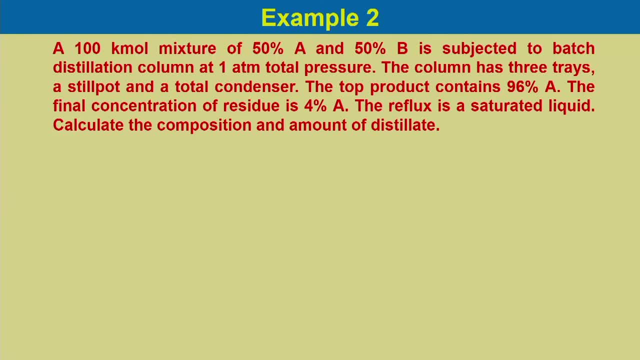 mixture of 50 mole percent D A and 50 mole percent D B. So 50 mole percent B is subjected to batch distillation column at 1 atmosphere pressure. the column has 3 trays, a steel pot and a total condenser. The top product contains: 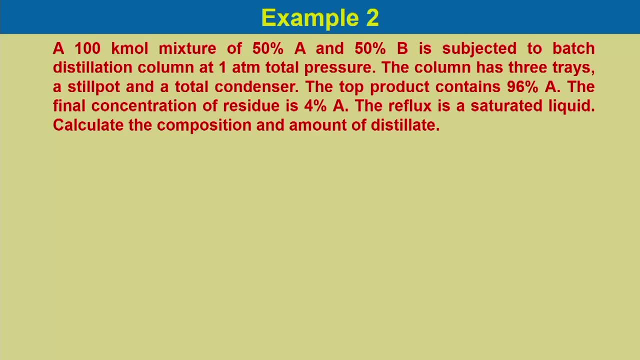 96 percent A. the final concentration of the residue is 4 percent A. the reflux is a saturated liquid. calculate the composition and amount of distillate. So that is one, and another one is the amount of top and bottom products, that is, know distillate. 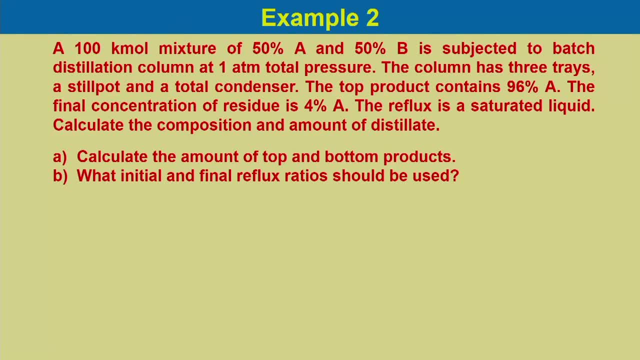 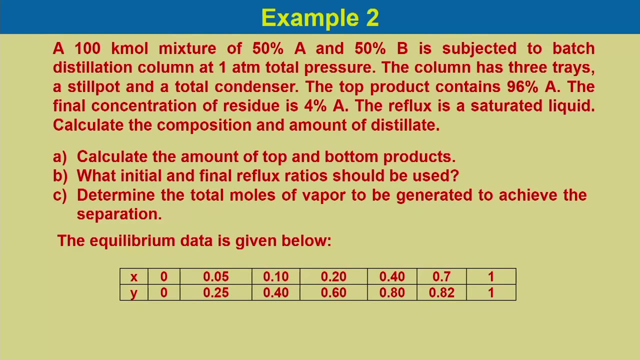 and the composition as well what initial and final reflux ratio should be used and determine the total moles of the vapour to be generated to achieve the separation. So to do that, these are the equilibrium data which are given: x and y. So this is the equilibrium data. So this is the equilibrium data which are given x. 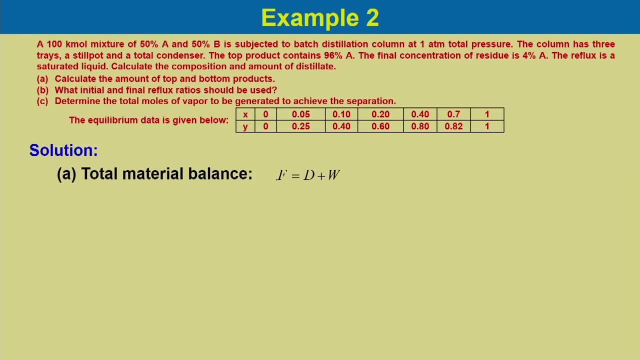 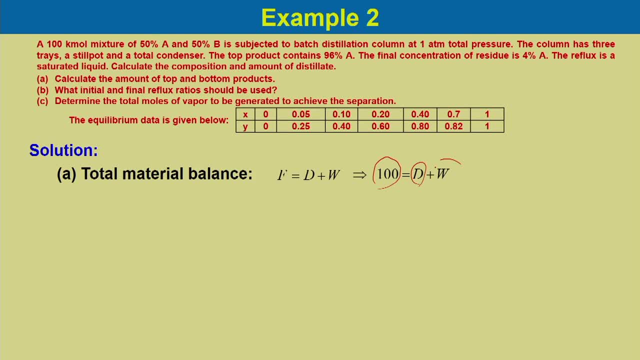 moles, So distillate. and the bottom. Now, if we do the component balance, it is F Z. f would be equal to the x, D plus W, that is D A by 1, contract of material balance D A. Now if we substitute the values: feed is 100 kilo mole having composition is 50 mole percent. 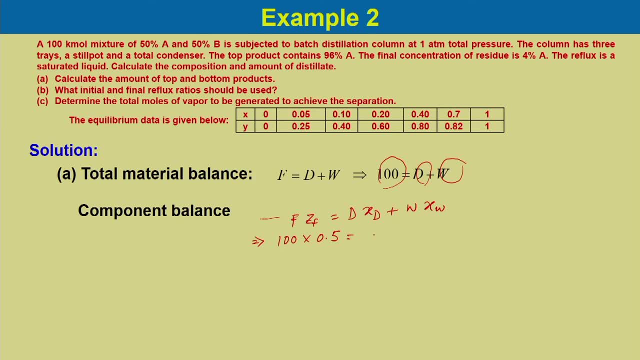 A, So it is 0.5- would be equal to distillate into its composition is 0.96, 96 percent A and the bottoms final composition W, into 0.04.. Now this would be 50, which is equal to 0.96. 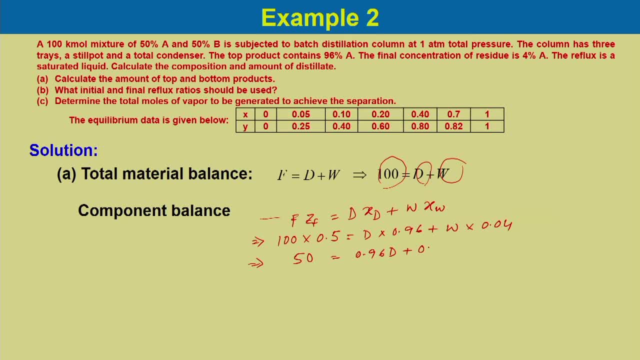 D plus 0.04 W. So if we substitute from the material balance, substitute W with 100 minus D, So it would be 0.96 D plus no 0.04 into 100 minus D. So in place of W we can substitute: 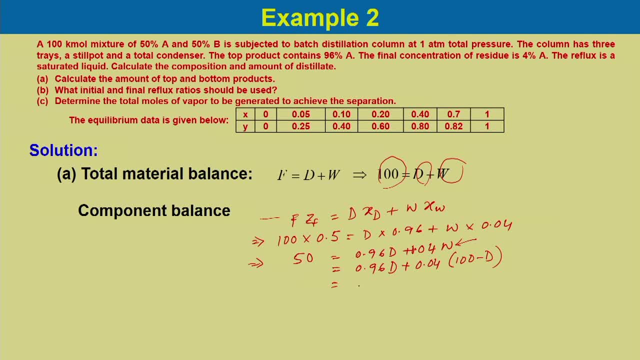 100 minus D. So essentially we will get 0.96 D plus 4 minus no 0.04 D. So from here we can write: no 0.92 D would be equal to 50 minus 4, which is 46, and we. 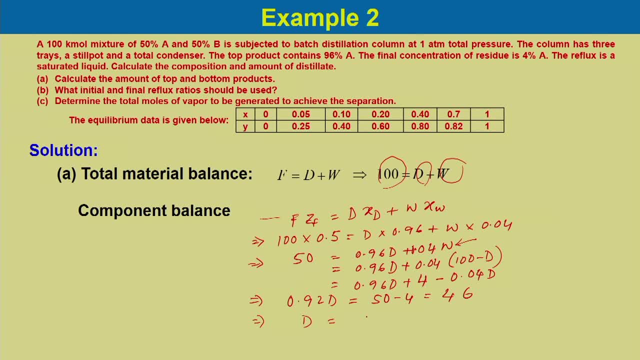 can obtain: D is equal to 46 divided by 0.92, which is equal to 50. So the distillate is is 50 kilo mole. So similarly we can obtain: from the total material balance: we can write: the D plus W would be 100. from here we can write: W would be 100 minus D, which is 100. 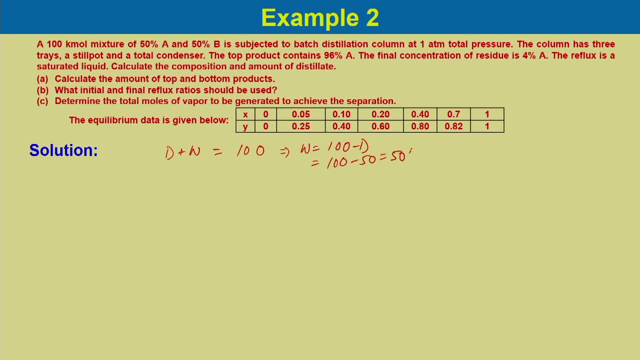 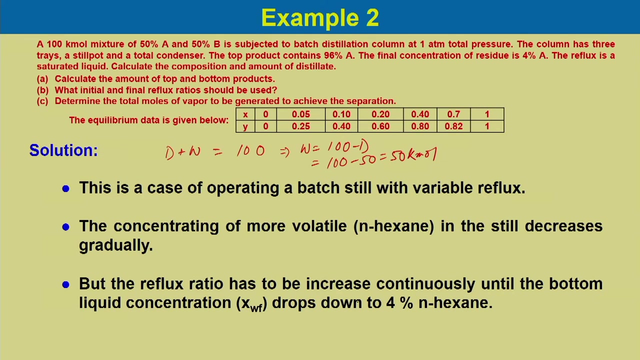 minus 50. So 50 K mole is the bottoms. So this is a case of operating a batch steel with variable reflux. the concentration of more volatile, that is, n hexane, in the steel decreases gradually and but the reflux has to be increased continuously until the bottom. 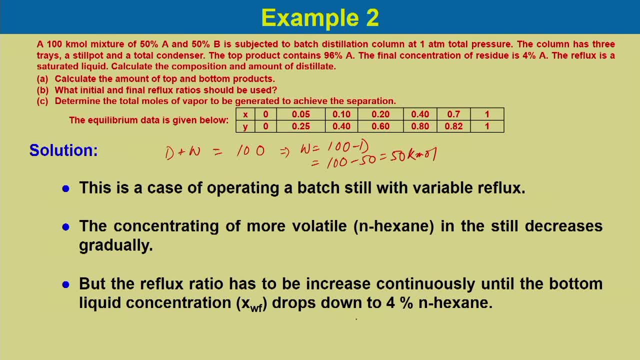 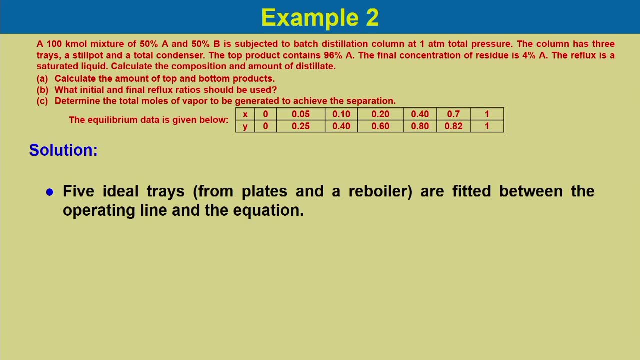 liquid concentration that is x, W, W drops down to 4 percent of n hexane. So there are 5 ideal trays from the plates and a reboiler which is, you know, fitted between the operating line and the equation. So you 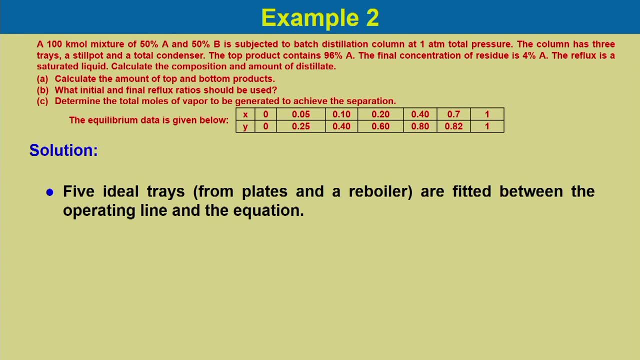 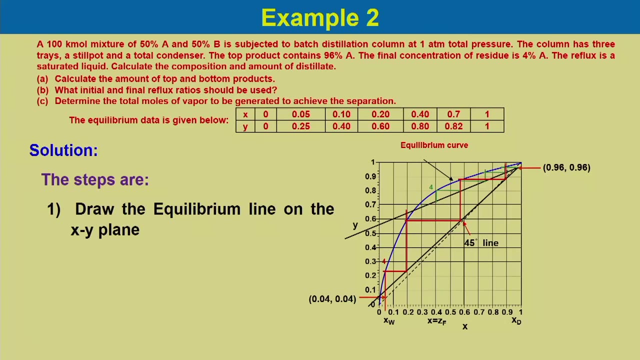 can see, there are 3 trays, one steel pot and one total condenser. So the overhead vapour concentration should always be 96 percent n hexane. Ok, So the steps to be followed here draw the equilibrium line with the data which are given. 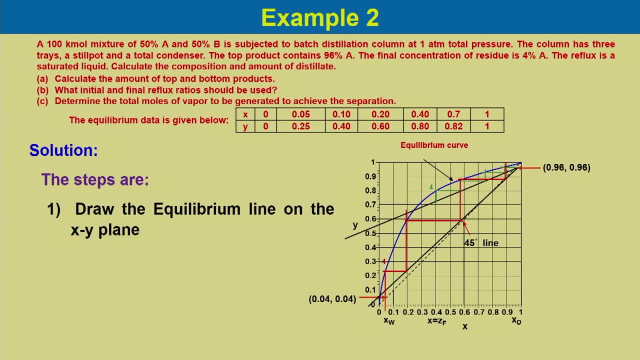 on the x y plane. So this is the blue line which is plotted over here- and then locate the point x d, x d, where x d is equal to 0.96.. So you can see, on the 45 degree diagonal, this is the point x d, x d. 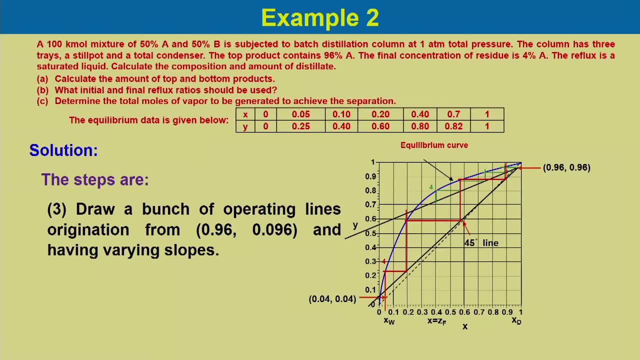 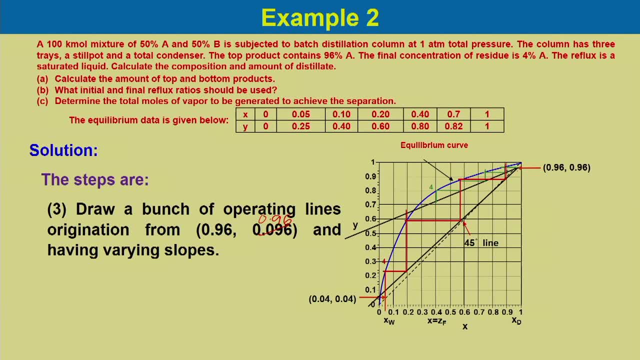 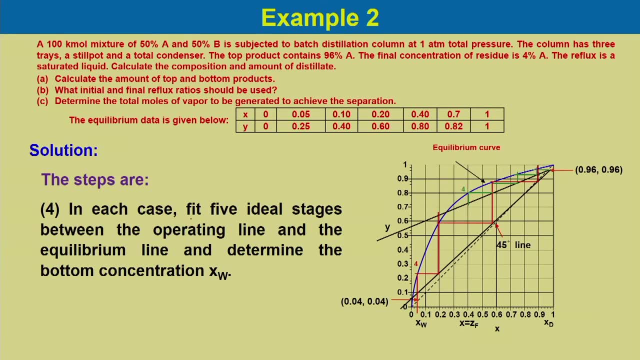 This is the number of operating lines starting from this point. In each case fit five ideal stages between the operating line and the equilibrium line and then determine the bottom concentration, that is xw. So for each of the operating line you are starting from xd. xd point and go to the equilibrium line and come vertically. 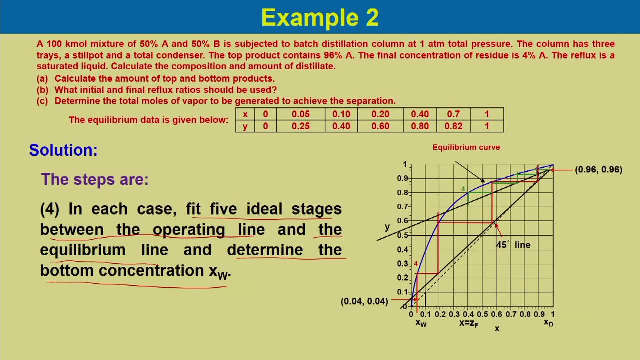 vertically to the operating line and then equilibrium, and vertical by staircase, no construction. as we did for the McCabe Thiele method, Similar method has to be followed to go up to the five ideal stages and then obtain the values in the x axis, the values of x, w, So each 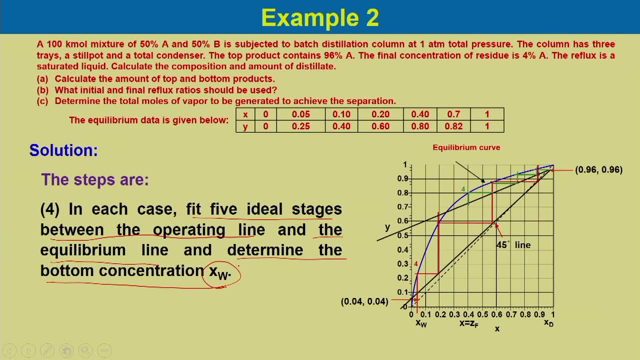 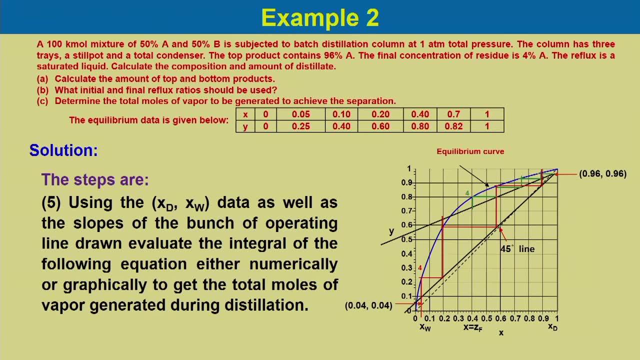 case, the bottom composition can be obtained with different reflux ratio Using the x, d and x w data, as well as the slopes of the bunch of operating line drawn. evaluate the integral of the following equation, either numerically or graphically, to get the total moles of vapour generated during distillation. So the equations which is known to you is: 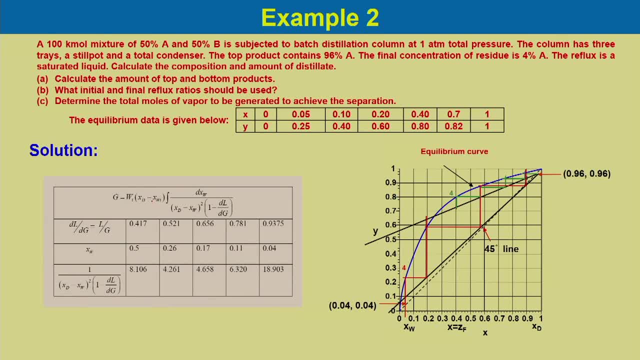 g would be equal to w i into x d minus x w i. integral d x w divided by x d minus x w square into 1 minus d L by d g. So this d l by d g is L by g. So this is the reflux. 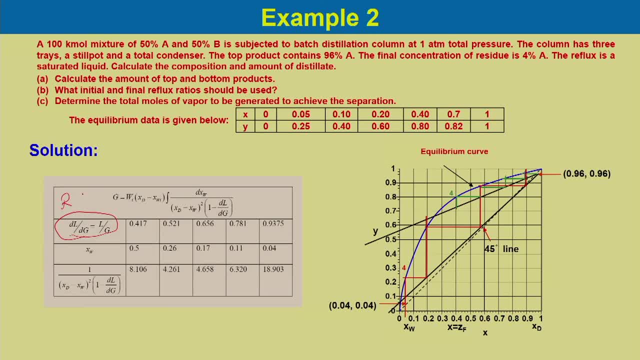 ratio we maintain or we vary. r is equal to L by g. So you can see initial composition is 0.5. with respect to X w, 0.5 we have to get for particular operating line having the reflux ratio L by G is 0.417.. So, with respect to 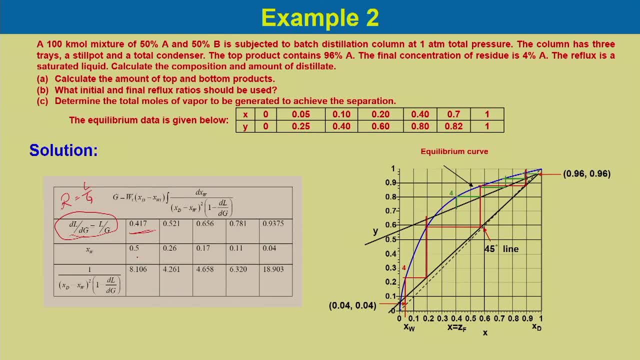 0.417, you will get X w is 0.5.. So once it is known, and then X d is fixed, 0.96 and 0.96.. So you can calculate from this: 1 by X d minus X w square into 1 minus d, l by d G, So d. 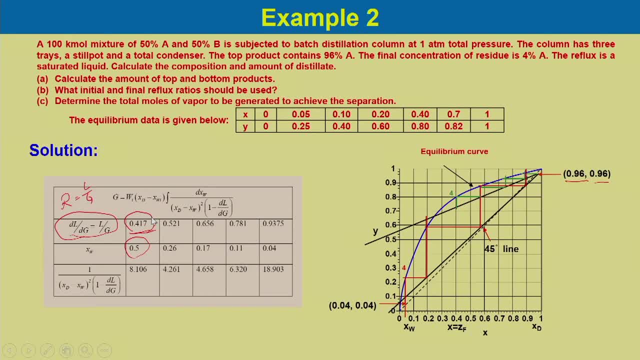 l by d, G is from here, from the reflux ratio you are varying and that for each case what you are doing, you will draw five ideal stages to obtain the bottom composition: X, w. So this is the range of reflux ratio. you could say that it is from length, 0.. perilous. 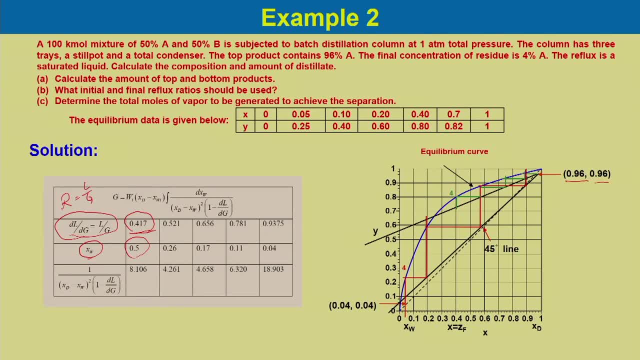 C, that is, the initial reflux ratio, is 0.417, corresponding to X. w is equal to 0.5 and finally you will obtain: X w is 0.4 percent in the residue, So 0.04, corresponding to the reflux. 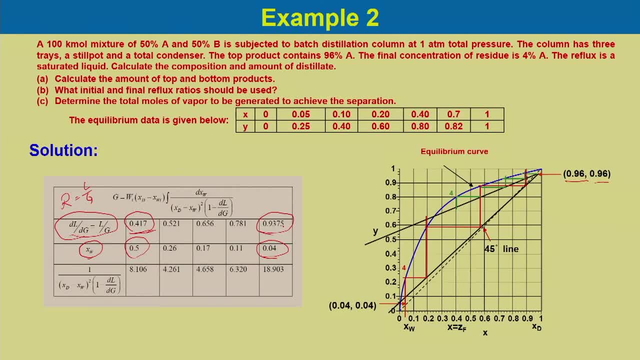 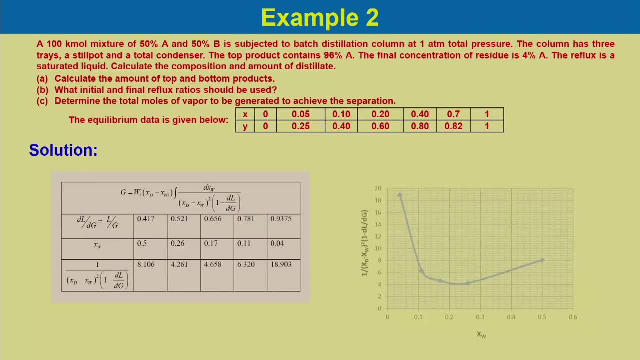 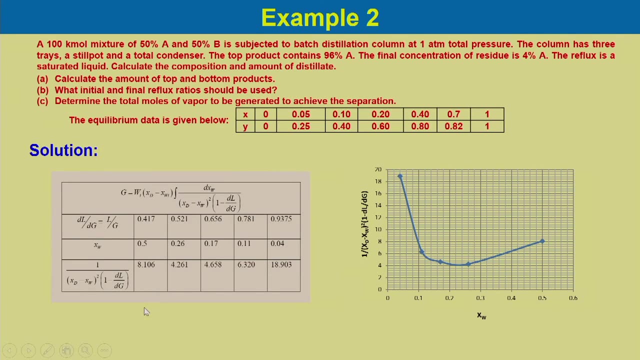 ratio, or L by g, is 0.9375.. So then you have this data. Now you plot this: 1 by X, d minus X w square into 1 minus d, L by d, g versus X w. If you plot, you will get this type of. 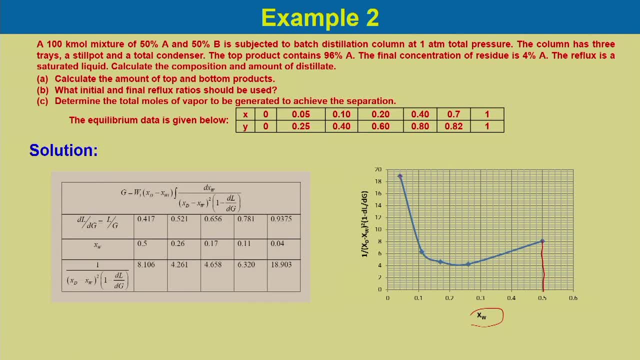 figure and this is from 0.04.. So this is up to from this 0.04.. So you need to calculate the area under this curve graphically and if you just get area under the curve So then you can just multiply with w? i into X d minus X w i, X d is known. 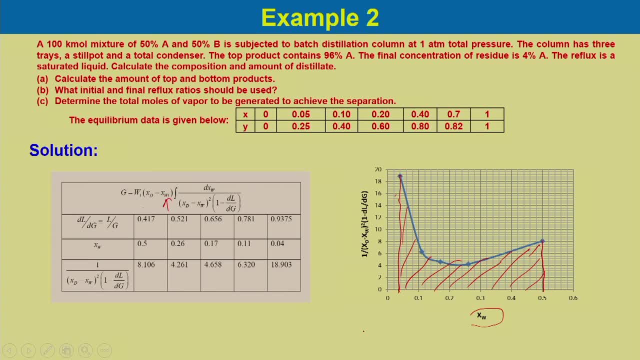 and X w i is also known to you. So the area under the curve from here you can calculate approximately 3 and you can calculate the total mole of vapour which would be generated would be equal to 100 into 0.96. is the distillate composition 0.96 X d minus X w i is you have? 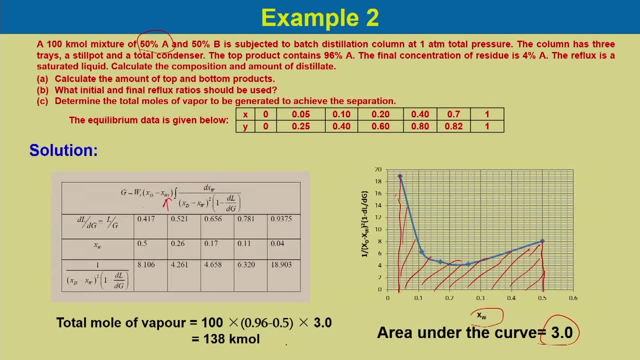 a 50 mole percent A. So X w i is 0.5 into the area under the curve which is 3.. So if you just multiply then it will give you 0.1.. So what does that fitness recover value look like according to the right hand side? So let us give some parameters to you. So that is veio, 1 square plus 1ем, to a point we8, you calculate 4 and then w is equal to health, ora 0.6. So this is our final reading, So this is the. 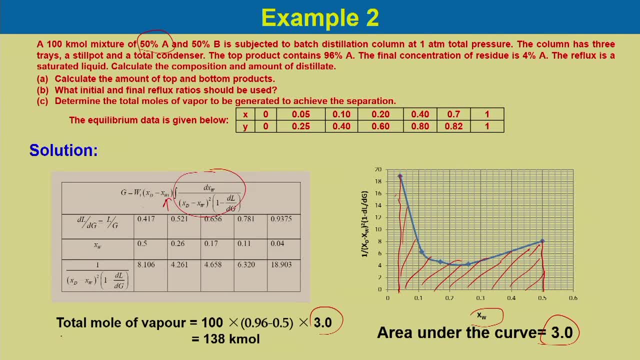 138 kilo mole. So the total mole of vapour which would be generated is 138 kilo mole. We have calculated the top and bottom products, the initial and final reflux ratio. this is the initial reflux ratio. it is W I. this is R I. initial reflux ratio corresponding to. 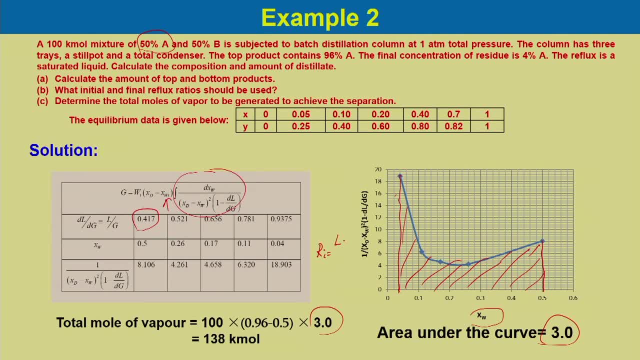 X W is equal to 0.5, is L I by G I and corresponding to the final reflux ratio, corresponding to X W is equal to 0.04, which is R F would be equal to L F by G F, So which is no 0.9375. 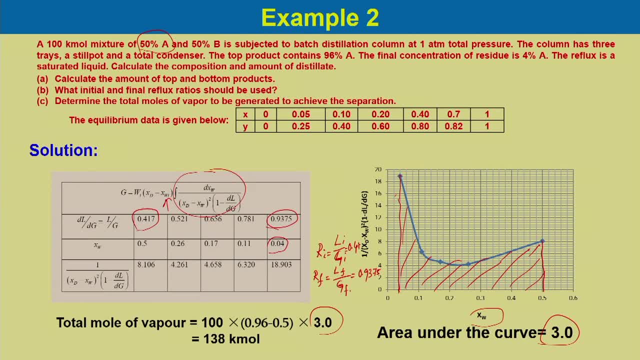 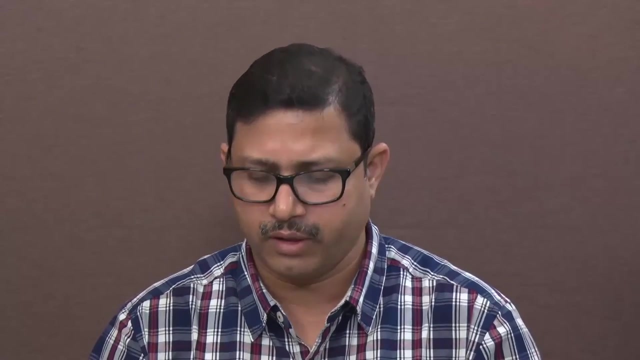 and this is no 0.5. And 417.. So the initial and final reflux ratio you can calculate and you can calculate the total mole of vapour which is generated for this distillation operation. So thank you for attending this lecture and we will continue. few more lectures to complete our 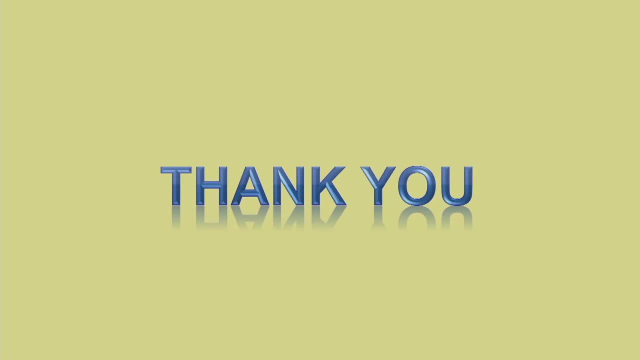 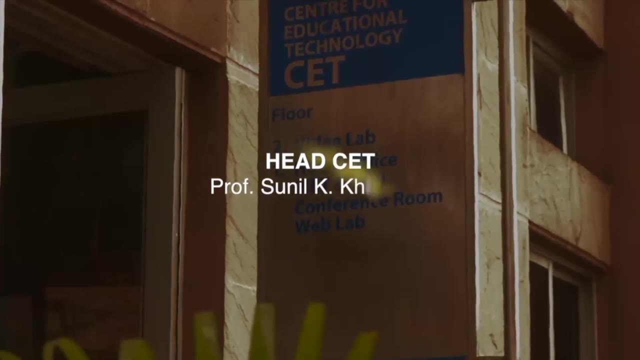 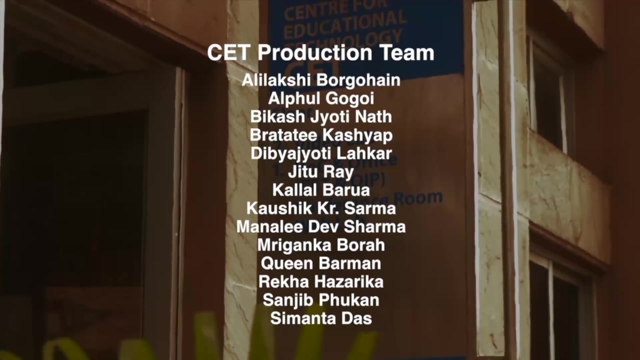 distillation operation. Thank you.